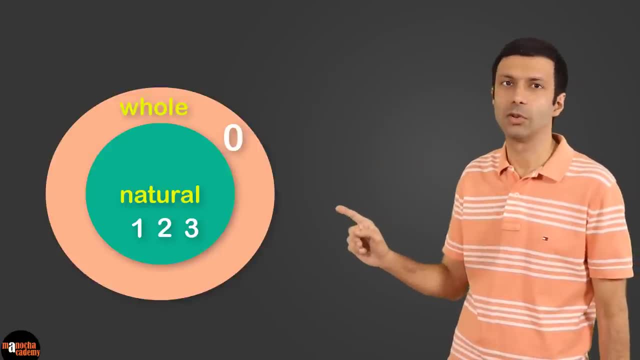 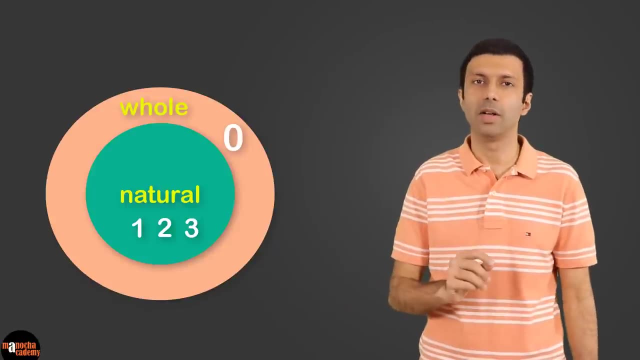 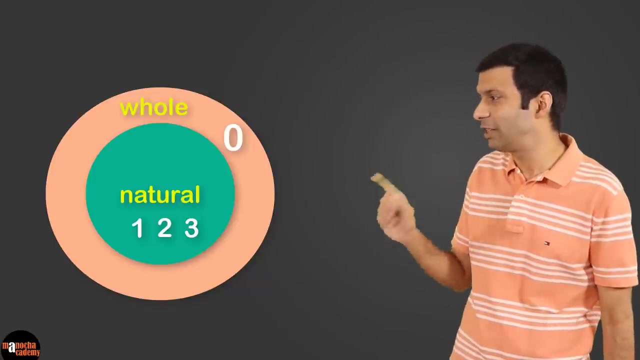 So we can draw the whole number circle around. the natural numbers, Integers include all the whole numbers and negative numbers such as minus one, two, three, four, five and minus one, minus two, minus three and so on. So we can draw the integer circle around. 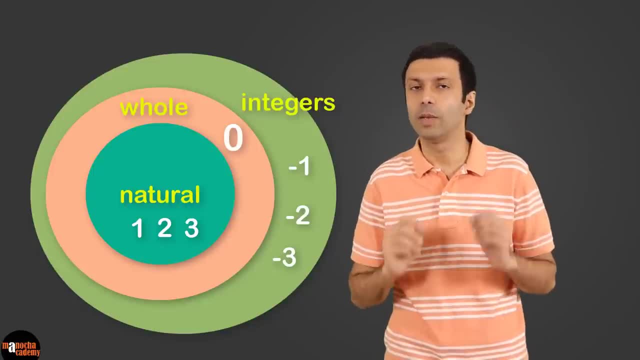 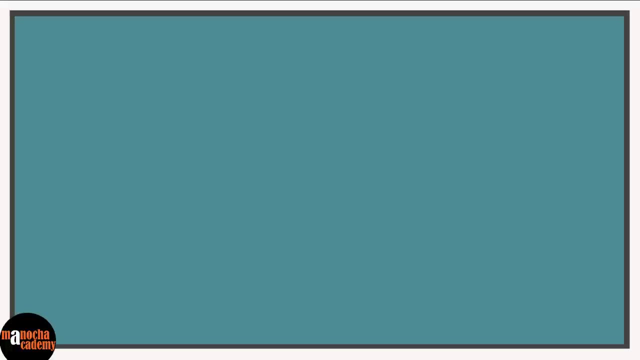 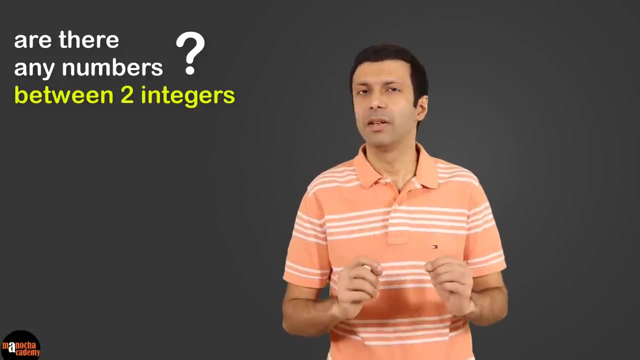 the whole numbers. One important thing for you to keep in mind is that zero is considered neither positive nor negative. Let's place the diagram we just did on our concept board. Now the question is: are there any numbers between any two integers, Let's say between: 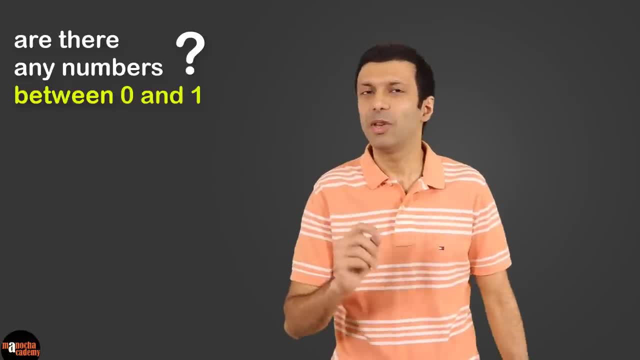 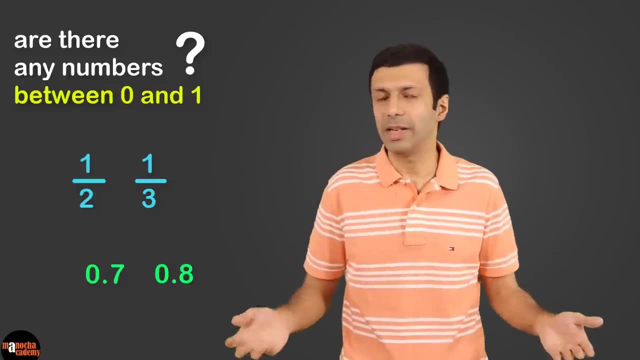 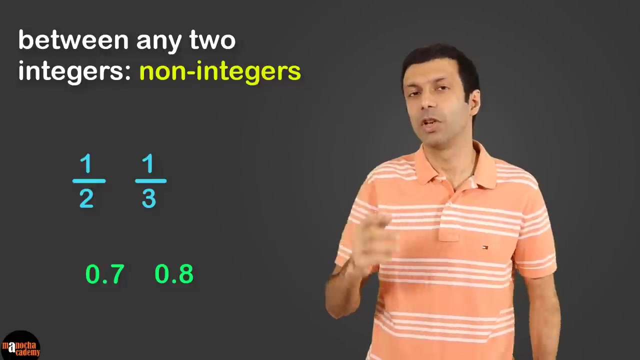 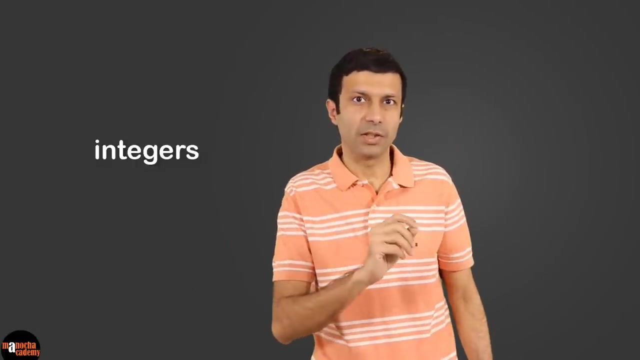 zero and one Yes, and we use them all the time, For example, half one-third, point seven, point eight. So between any two integers you have these non-integer numbers, which are known as fractions or decimals, And this entire set of integers and fractions and decimals. 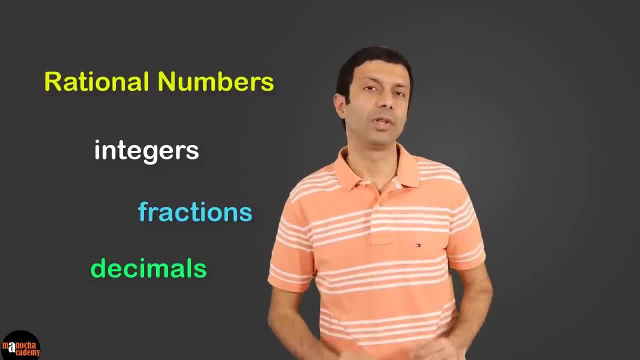 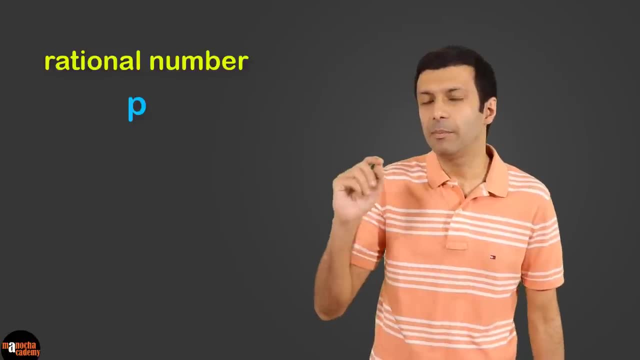 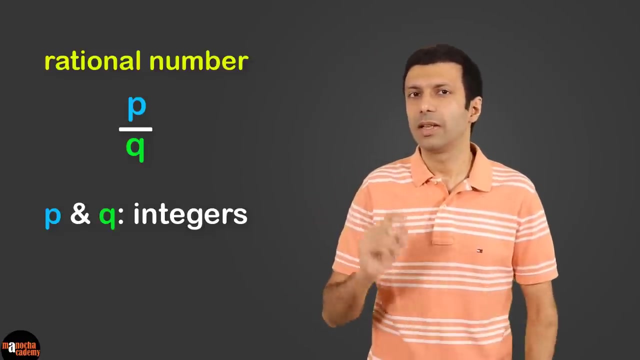 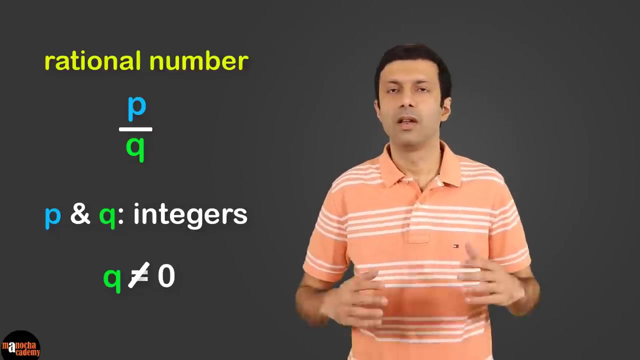 are called rational numbers And they are denoted by the letter Q. Any rational number can be written as a fraction: P by Q, where P and Q are integers. The only restriction is that Q should not be zero, since division by zero is undefined. Now is the natural number three also a rational? 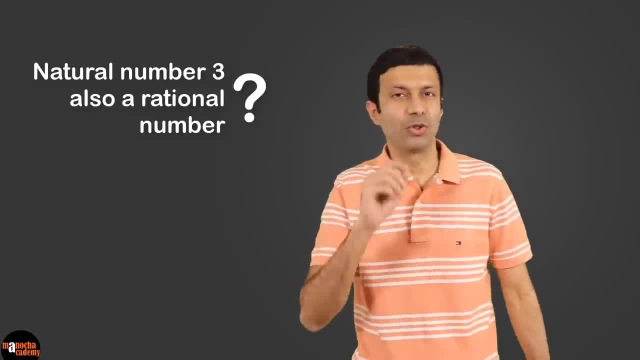 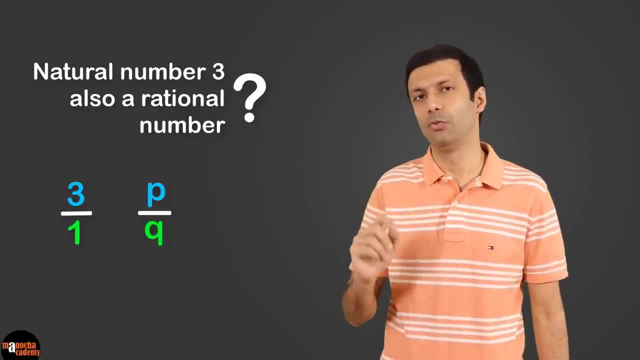 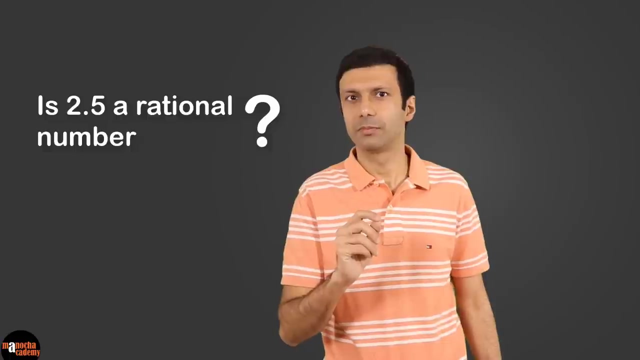 number, What do you think? So three can be written as Three by one. It can be written as a fraction in a P by Q form. So three is also a rational number. Now, what about 2.5?? So we can write it as 25 by 10.. And if you simplify the fraction, 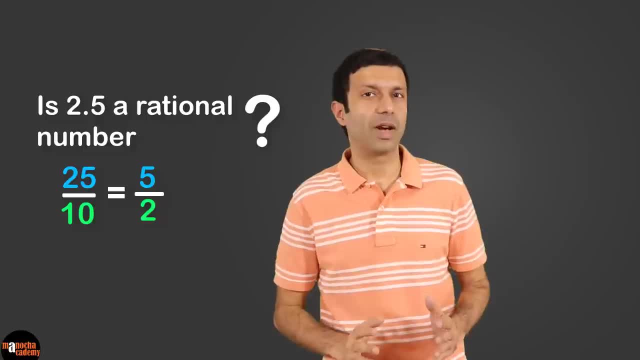 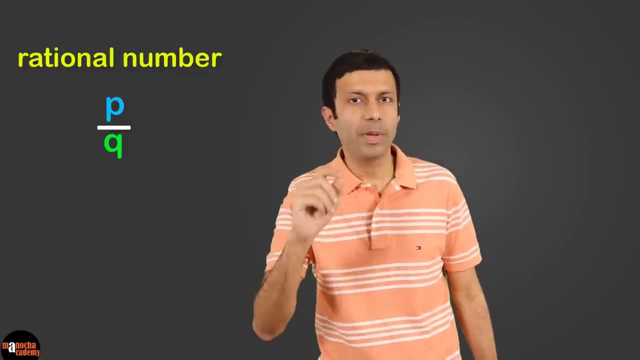 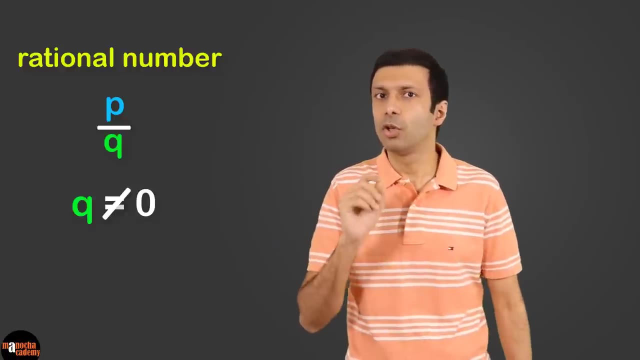 you get 5 by 2. So 2.5 is also a rational number. So any rational number can be expressed in a P by Q form, That is, in this fraction form. The only restriction is Q should not be equal to zero, And typically 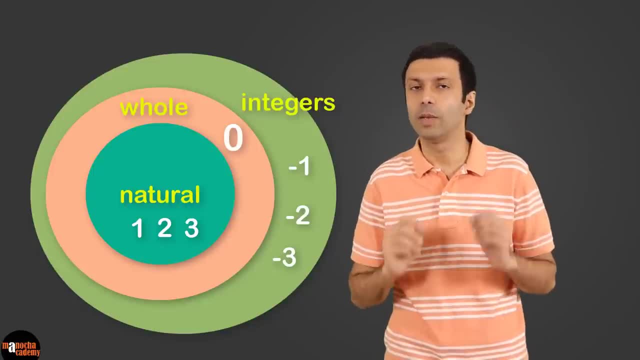 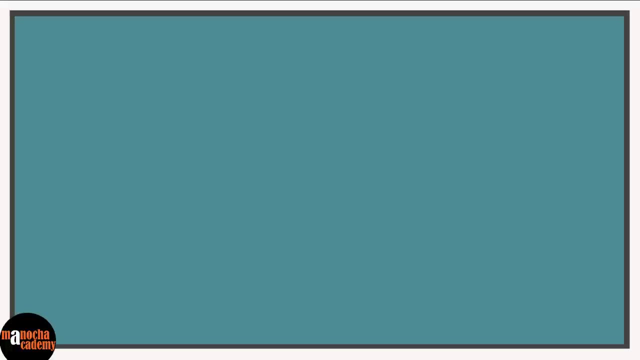 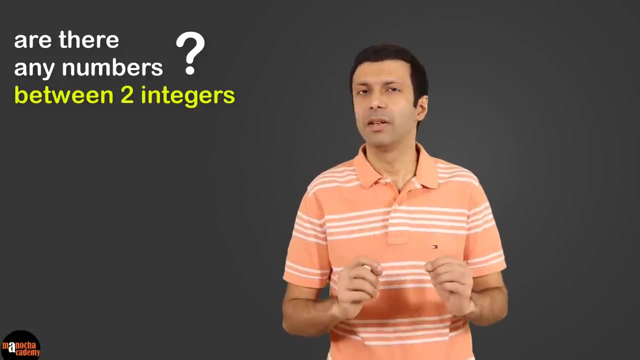 the whole numbers. One important thing for you to keep in mind is that zero is considered neither positive nor negative. Let's place the diagram we just did on our concept board. Now the question is: are there any numbers between any two integers, Let's say between: 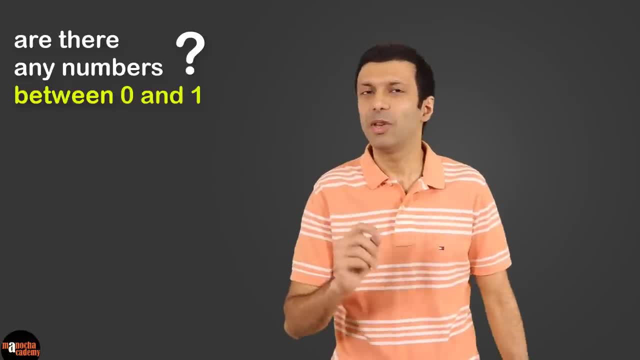 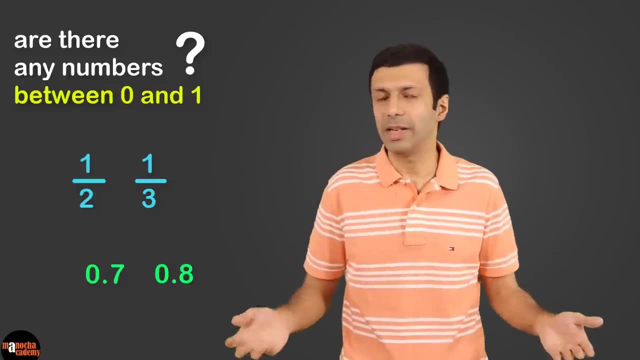 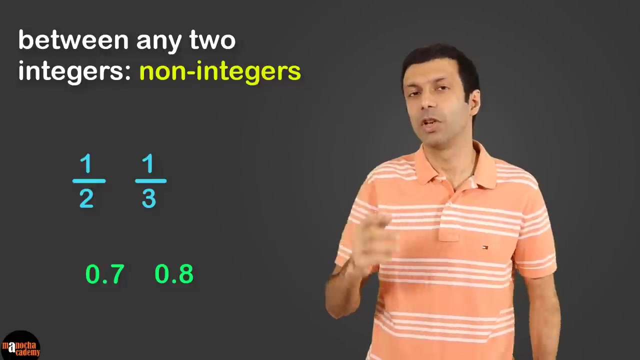 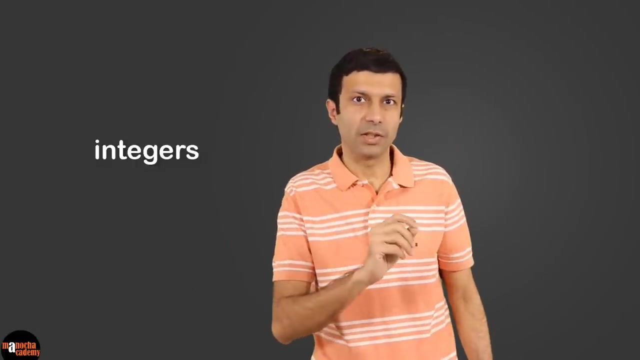 zero and one Yes, and we use them all the time, For example, half one-third, point seven, point eight. So between any two integers you have these non-integer numbers, which are known as fractions or decimals, And this entire set of integers and fractions and decimals. 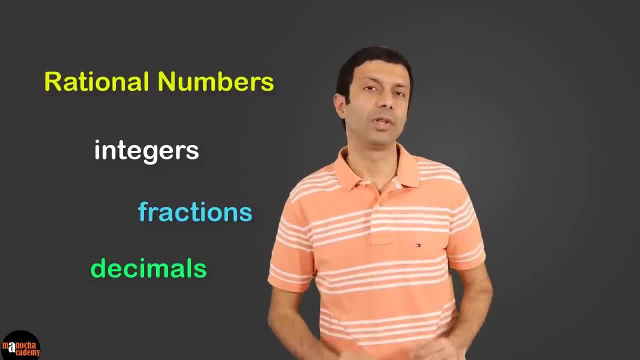 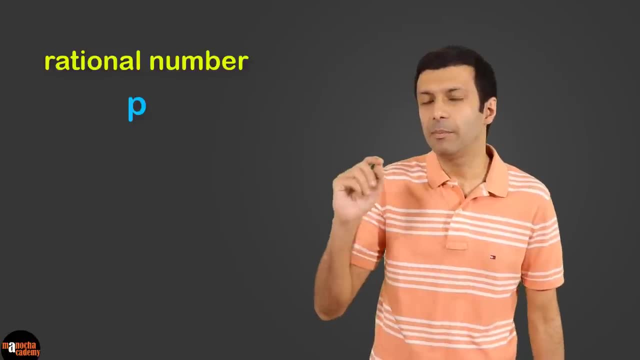 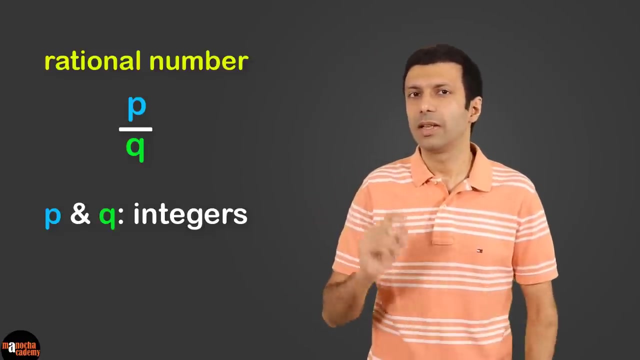 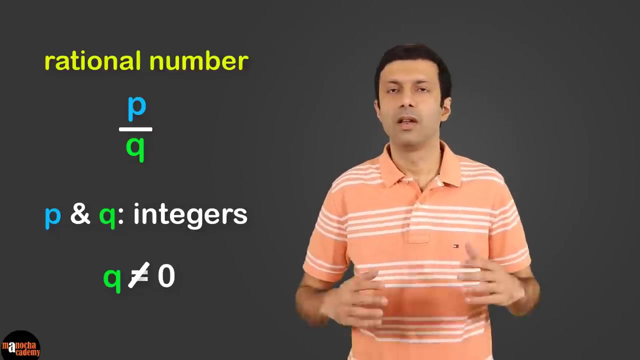 are called rational numbers And they are denoted by the letter Q. Any rational number can be written as a fraction: P by Q, where P and Q are integers. The only restriction is that Q should not be zero, since division by zero is undefined. Now is the natural number three also a rational? 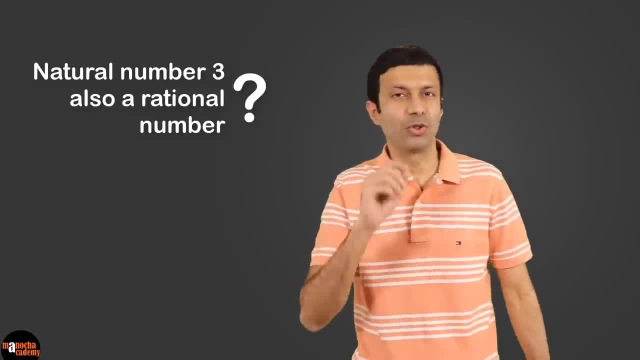 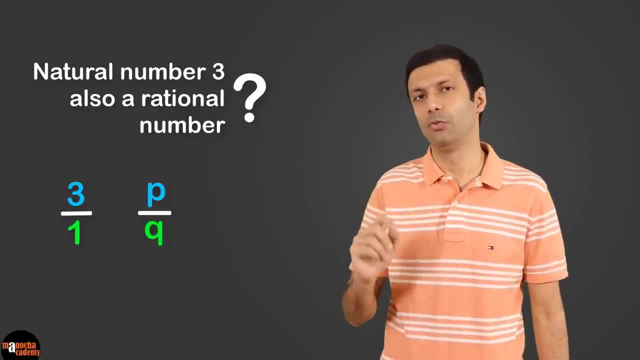 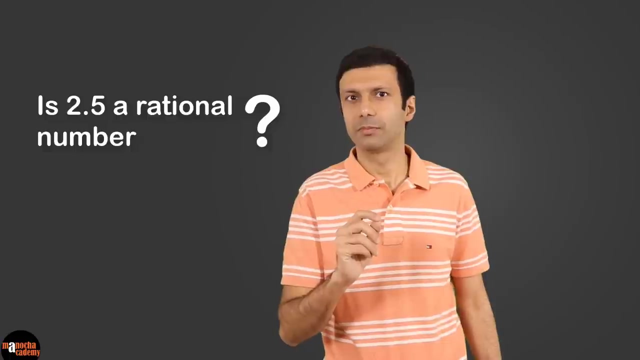 number, What do you think? So three can be written as Three by one. It can be written as a fraction in a P by Q form. So three is also a rational number. Now, what about 2.5?? So we can write it as 25 by 10.. And if you simplify the fraction, 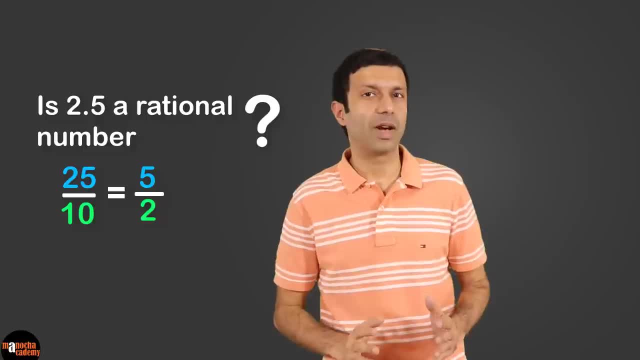 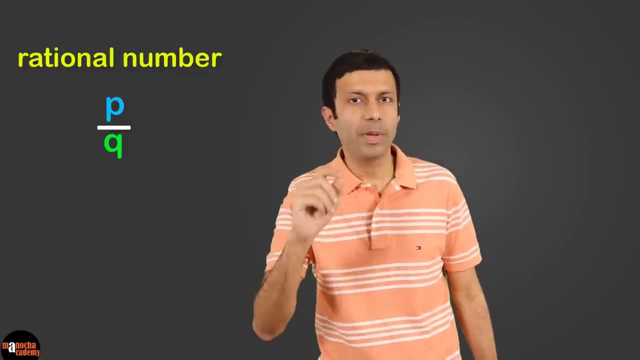 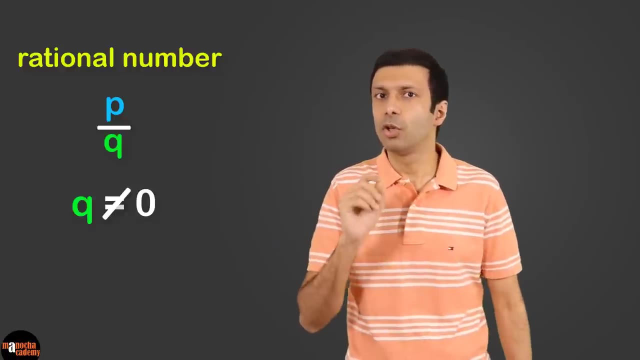 you get 5 by 2. So 2.5 is also a rational number. So any rational number can be expressed in a P by Q form, That is, in this fraction form. The only restriction is Q should not be equal to zero, And typically 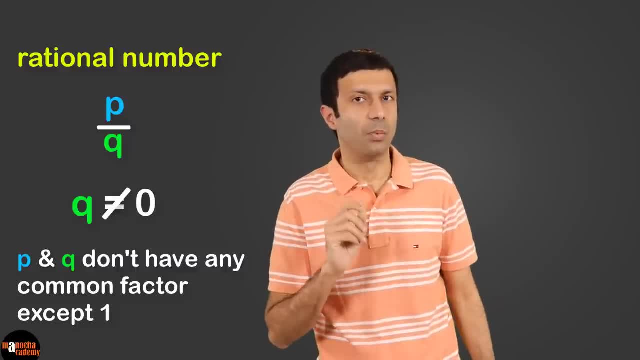 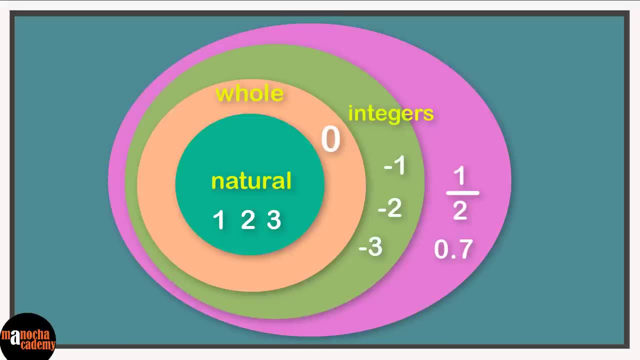 P and Q don't have any common factor except one, So we write the fraction in its simplified form. Let's add the non-integers to our set diagram. The integers and non-integers, that is fractions and decimals together, are called rational numbers. 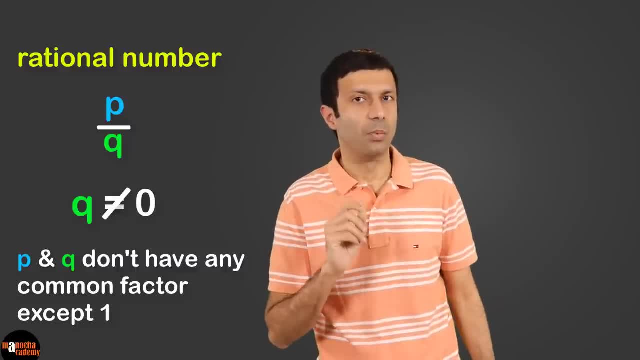 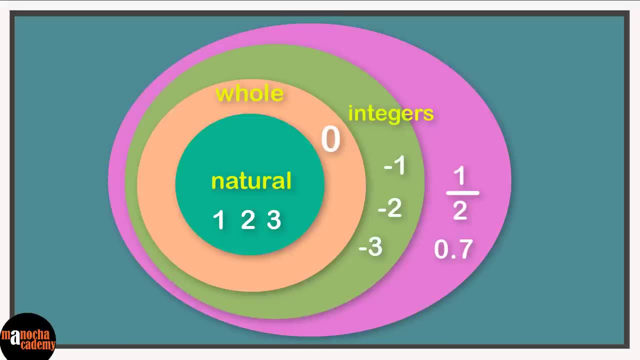 P and Q don't have any common factor except one, So we write the fraction in its simplified form. Let's add the non-integers to our set diagram. The integers and non-integers, that is fractions and decimals together, are called rational numbers. 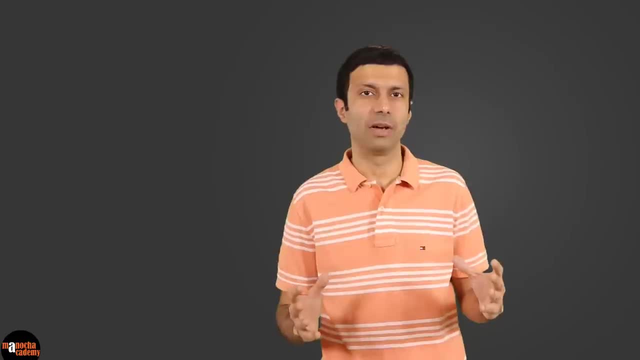 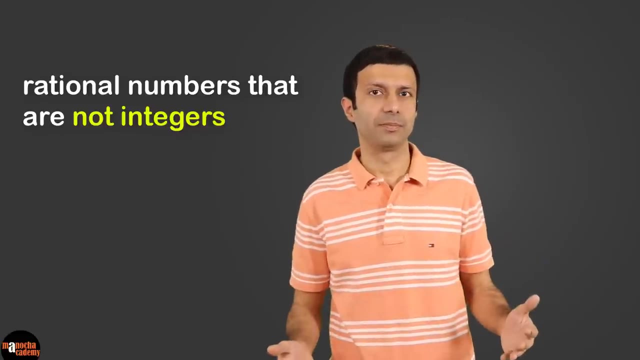 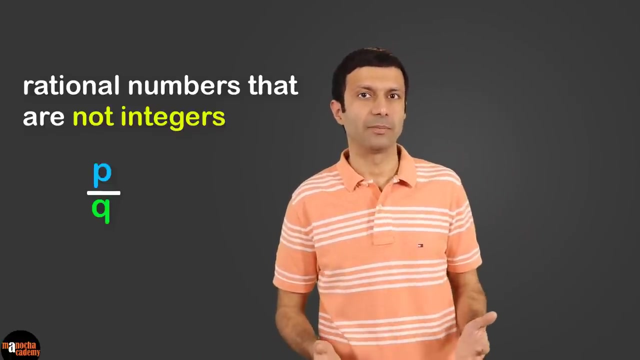 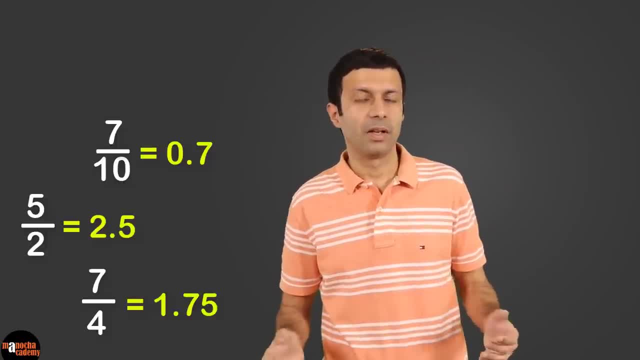 7 by 2 is 2.5.. So 7 by 2 is 2.5.. So 7 by 2 is 2.5.. So 7 by 2 is 2.5.. 7 by 4 is 1.75.. These are all examples of terminating decimal numbers. That is the. 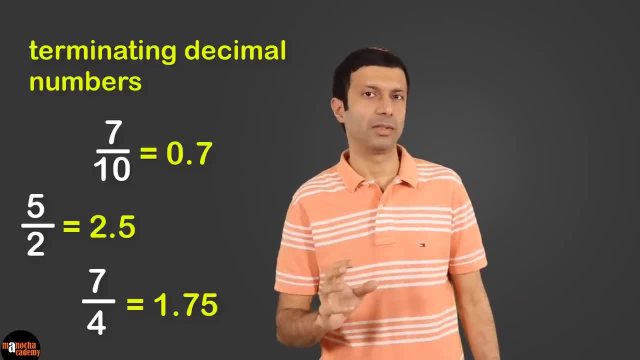 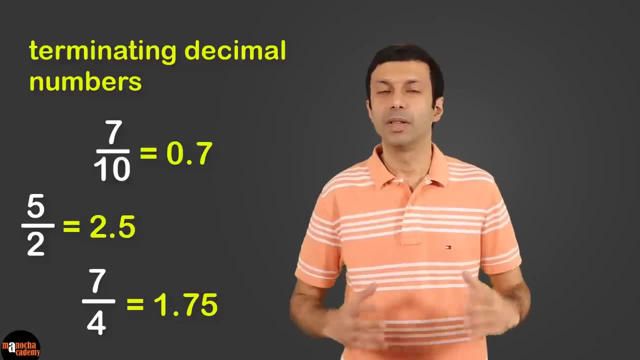 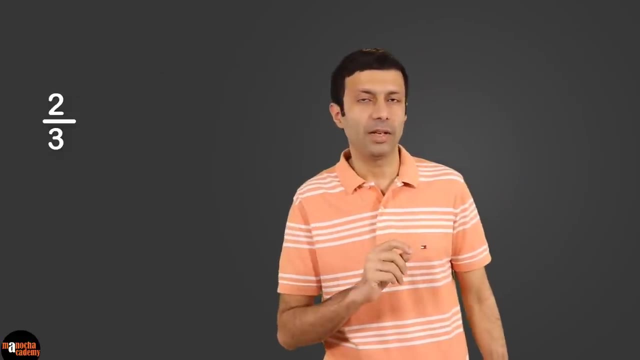 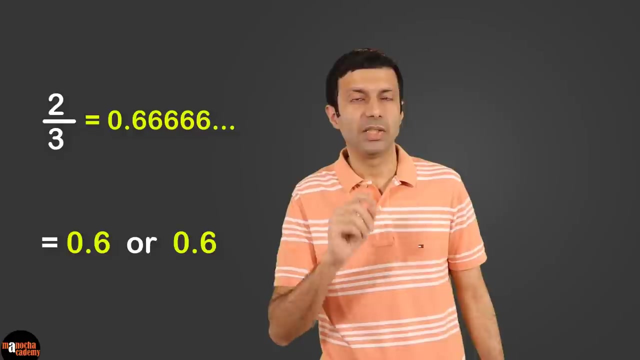 decimal digits stop or terminate after a point, Because on dividing by the denominator, the remainder is 0.. But there are other fractions which, on dividing, don't terminate. For example, 2 by 3 is 0.67.. six, six, six, six, and it just goes on. so we write it as 0.6 with a dot or a line. 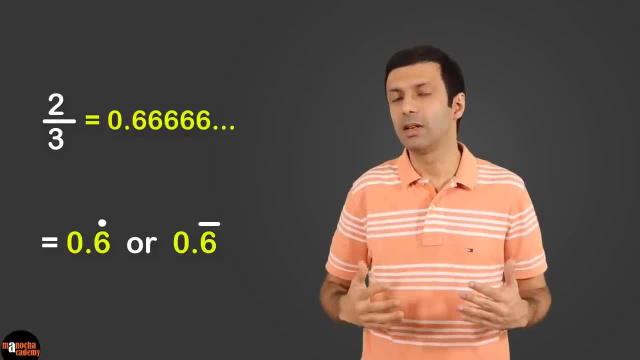 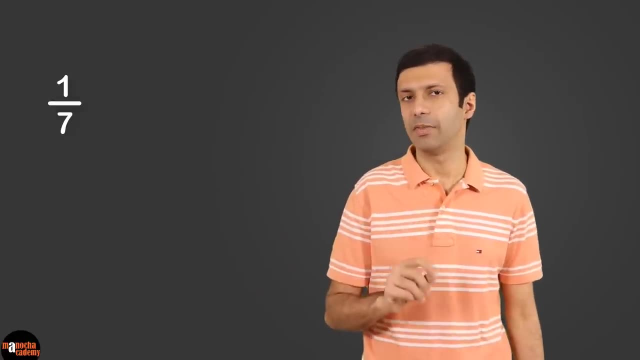 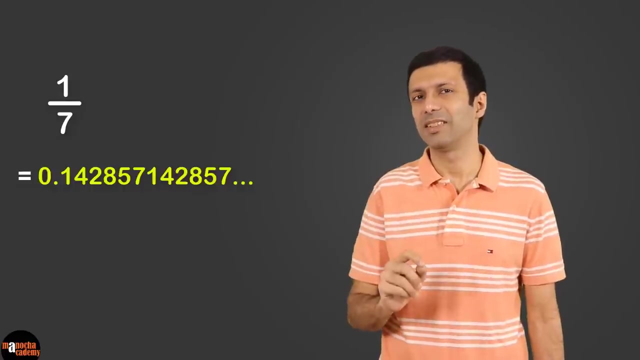 on top to represent that the digit 6 is recurring, which means repeating. let's take another example: 1 by 7. so if you look at the answer here, can you see the repeating pattern. that's right, it's zero point one, four, two, eight, five, seven. 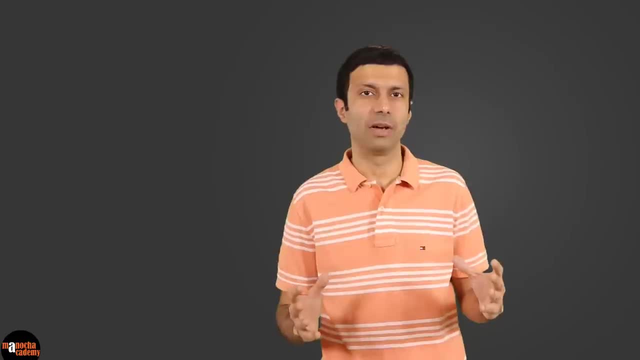 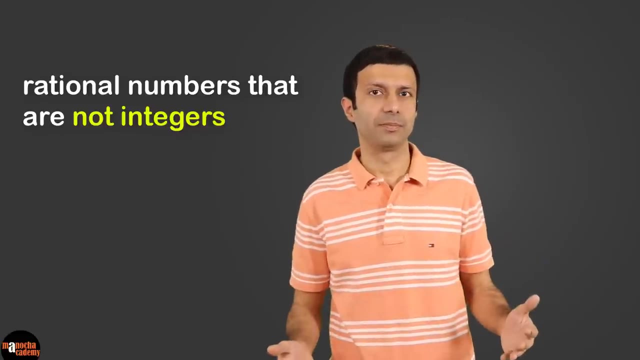 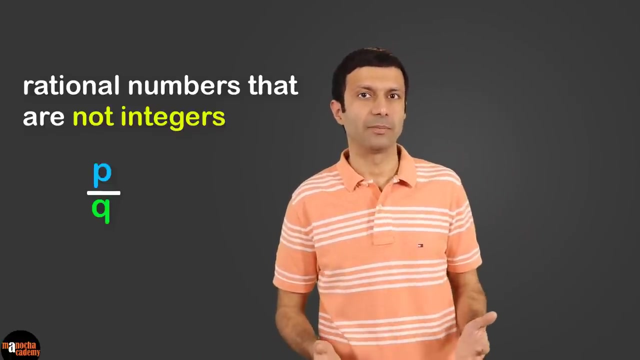 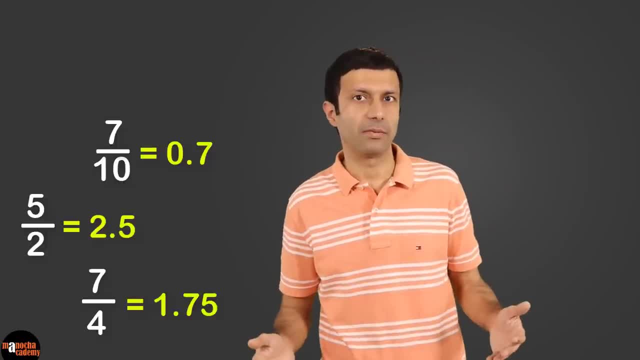 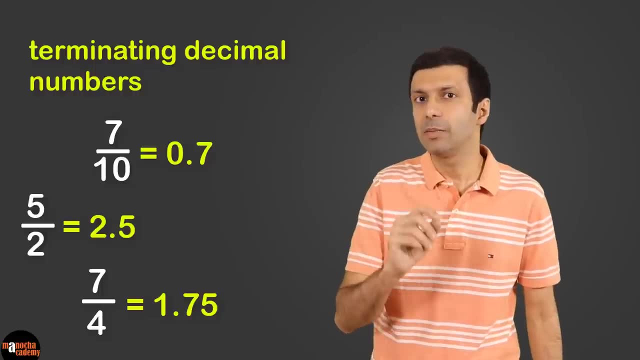 7 by 2 is 2.5.. So 7 by 3 is 2.5.. 7 by 4 is 1.75.. These are all examples of terminating decimal numbers, That is, the decimal digits stop or terminate after a point, Because on. 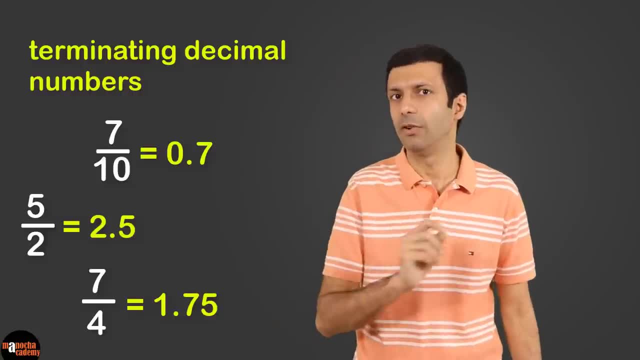 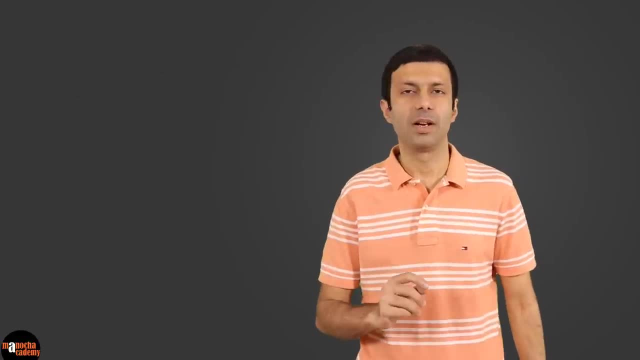 dividing by the denominator, the remainder is 0.. But there are other fractions which, on dividing, don't terminate, For example 2 by 3 is 0.65, which on dividing don't terminate, For example, 2 by 3 is 0.67, which, What about? 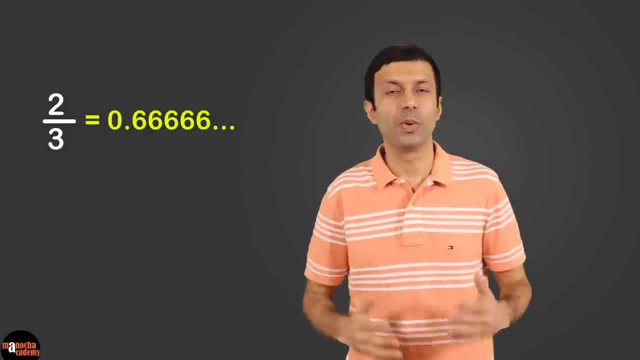 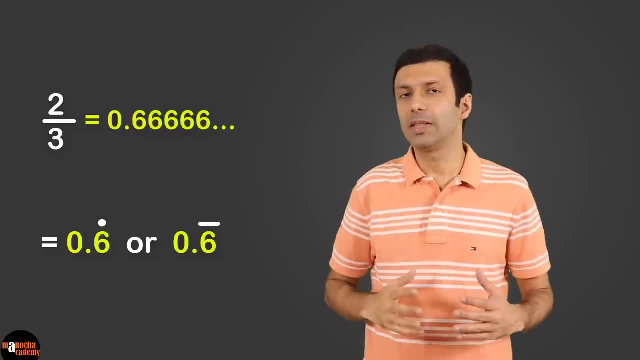 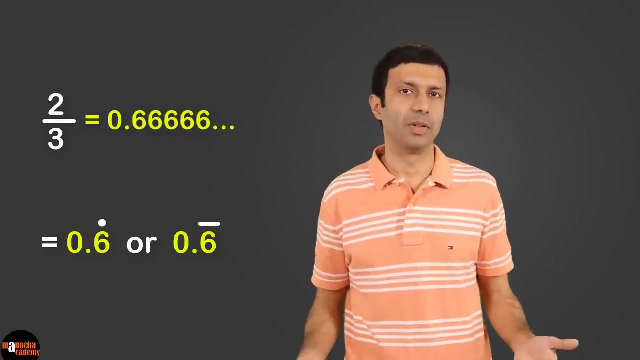 six, six, six and it just goes on. so we write it as 0.6, with a dot or a line on top to represent that the digit 6 is recurring, which means repeating. let's take another example: 1 by 7. so if you look at the answer here, can you see the 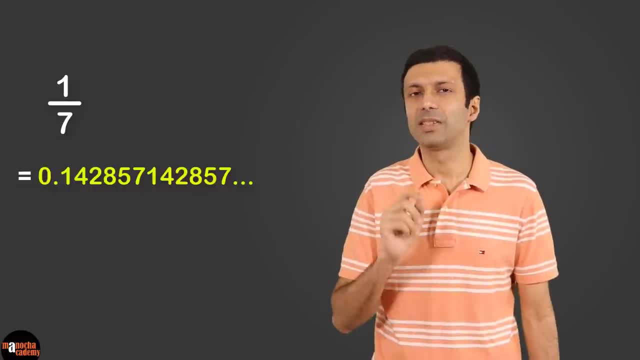 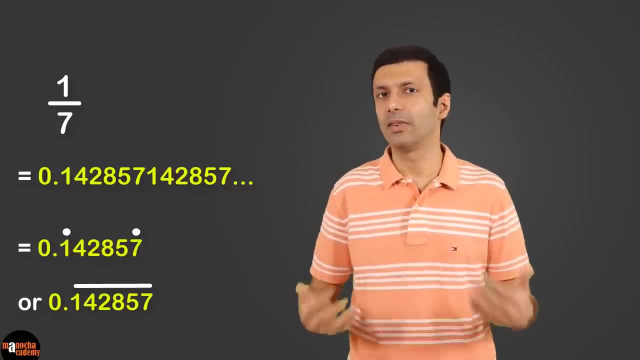 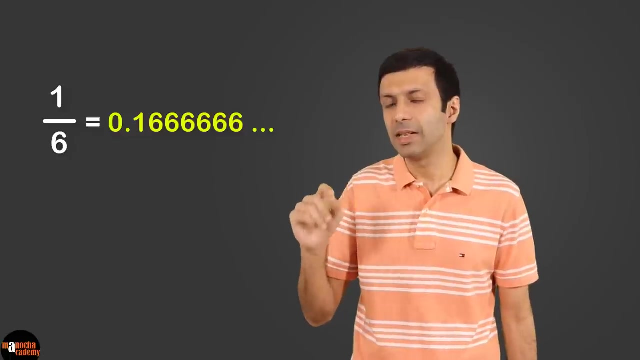 repeating pattern. that's right. it's 0 point 1, 4, 2, 8, 5, 7, recurring. let's take a look at another example: 1 by 6, so that's going to be 0 point 1, 6, 6, 6, 6 and it. 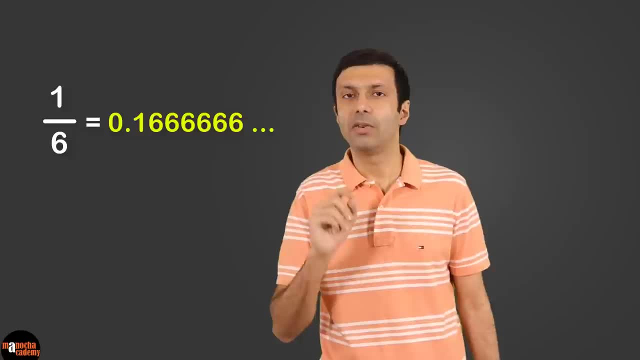 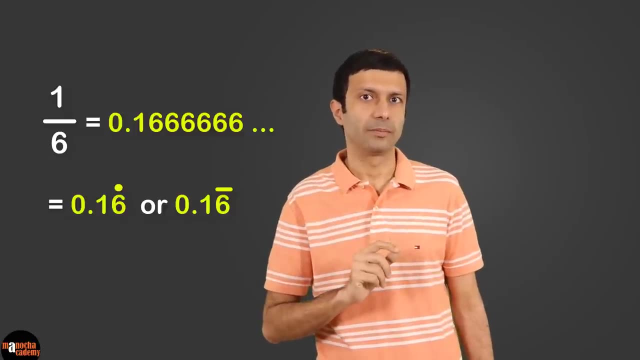 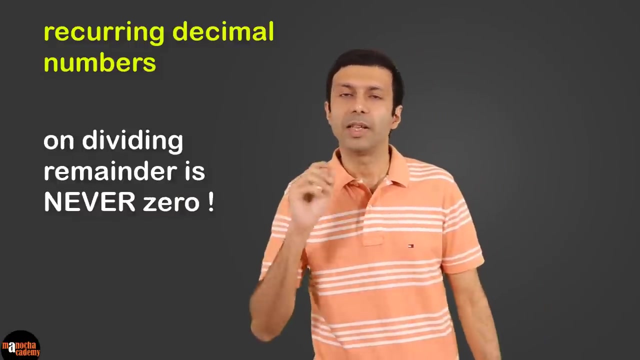 just keeps repeating. but notice that we write it with a dot or a bar only on top of 6, because only the 6 is repeating. so these are called recurring decimal numbers, where on dividing by the denominator, the remainder is never 0 and the digits in the quotient keep. 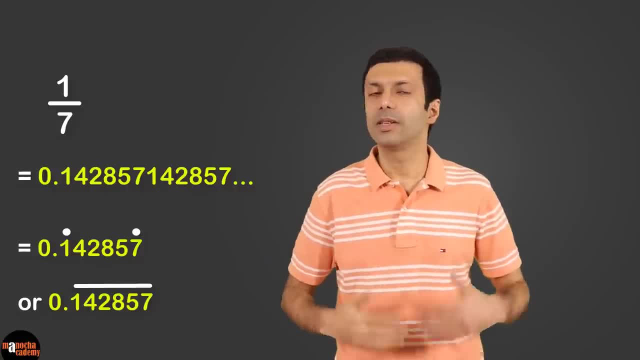 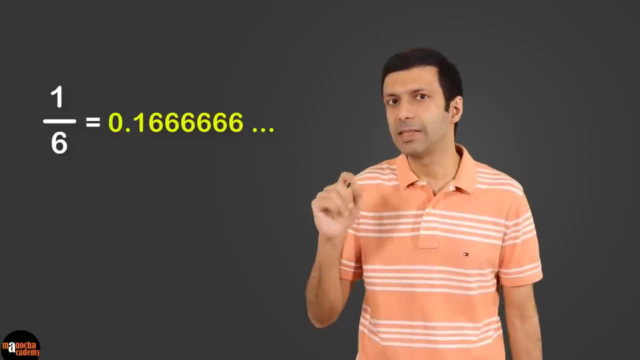 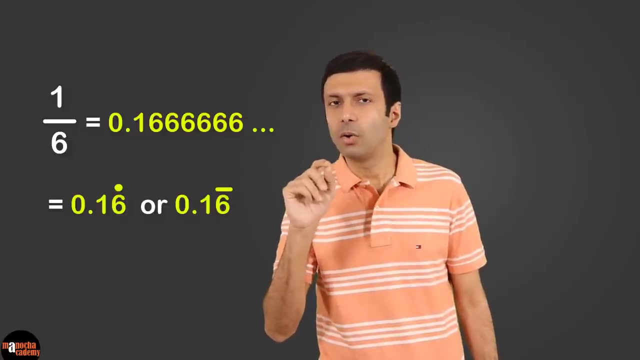 recurring. let's take a look at another example: 1 by 6, so that's going to be zero point one. six, six, six, six and it just keeps repeating. but notice that we write it with a dot or a bar only on top of 6, because only the 6 is repeating. so 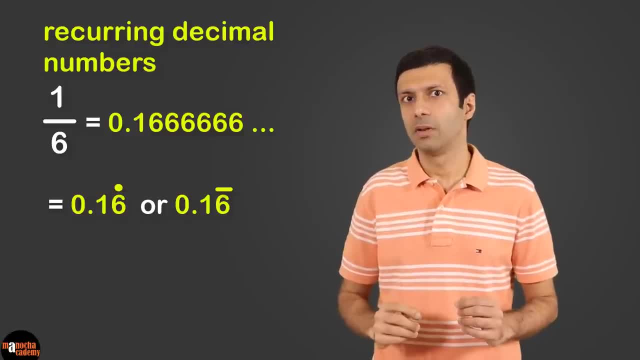 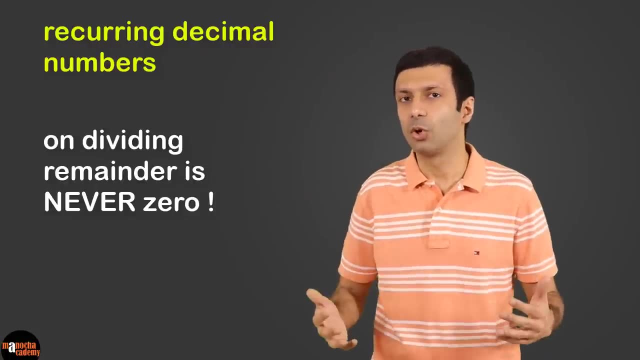 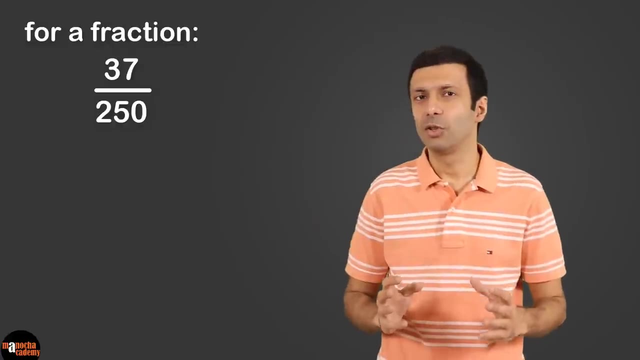 these are called recurring decimal numbers, where, on dividing by the denominator, the remainder is never 0 and the digits in the quotient keep repeating. if you take any fraction, how do you determine that on division you're going to get a terminating decimal number or a recurring decimal number of? 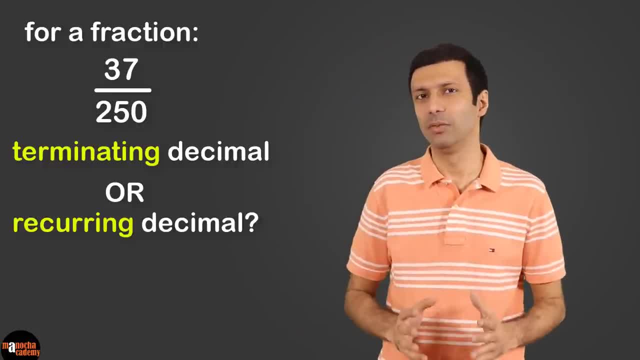 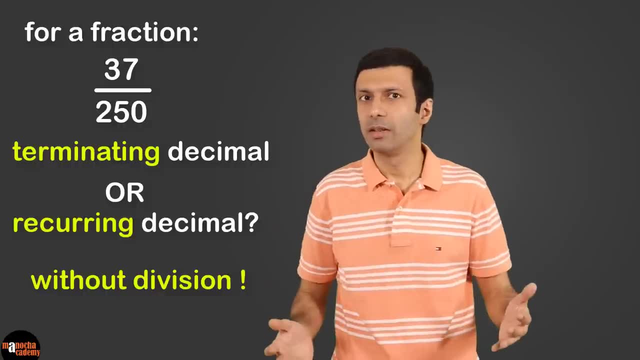 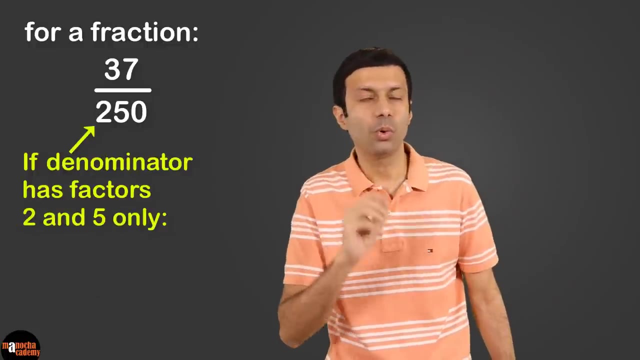 course, one simple way is to actually do the division, but there's another trick where you don't need to do it divide. now, what's the trick? you need to take a look at the denominator, and if the denominator has factors of 2 and 5, only then you're going to get a 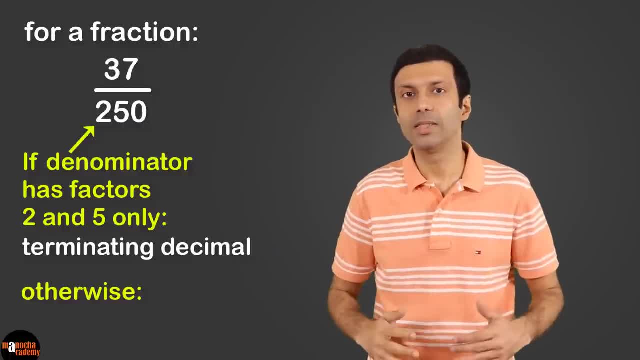 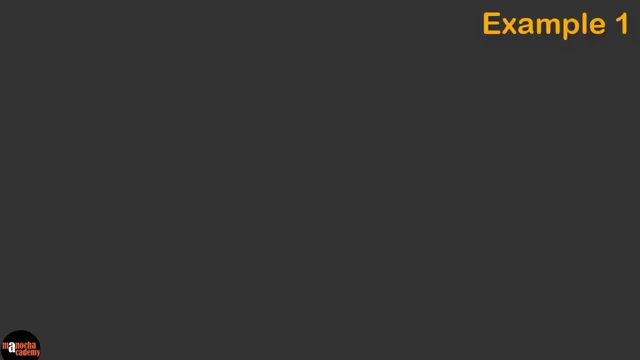 terminating decimal number, otherwise it's going to be a recurring decimal number. let me pull up some examples to illustrate this. let's start with the example of 7 by 4. now what are the factors of the denominator 4? it's 2 into 2. now our goal is to convert the denominator into multiples. 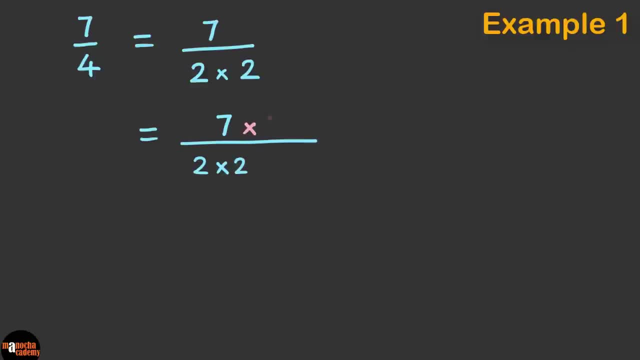 of tens. so I'm going to multiply 5 into 5 in the numerator and in the denominator. so I get 175 by 100, that's 1.75. so this is a terminating decimal number. but if we take 37 by 150. so what are the factors of the denominator? 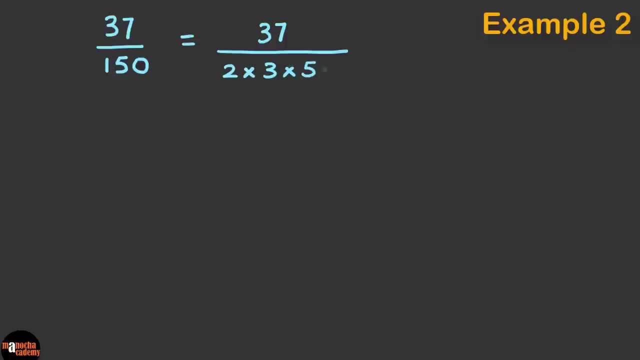 they are 2 into 3, into 5 into 5, and if you divide we get 0.24666 and so on. so this is a recurring decimal number. and why is that? because if you carefully look at the factors in the denominator, you can see that there's a 3 there, for 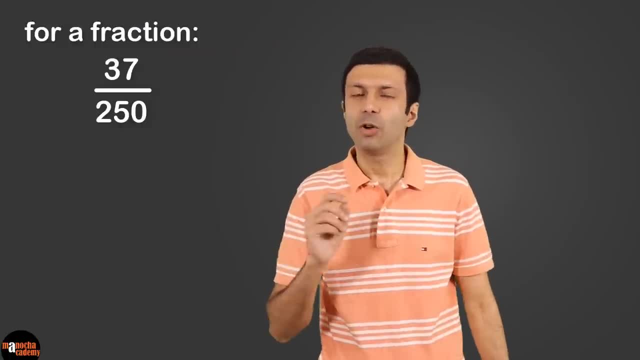 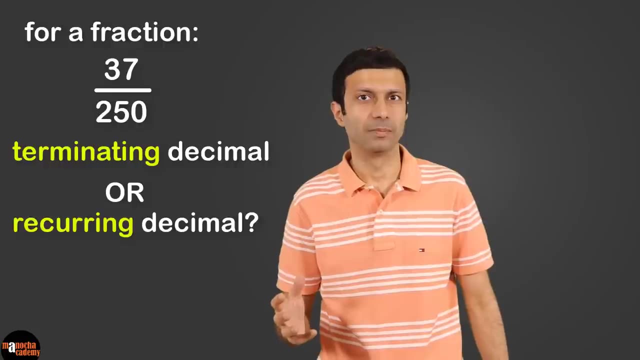 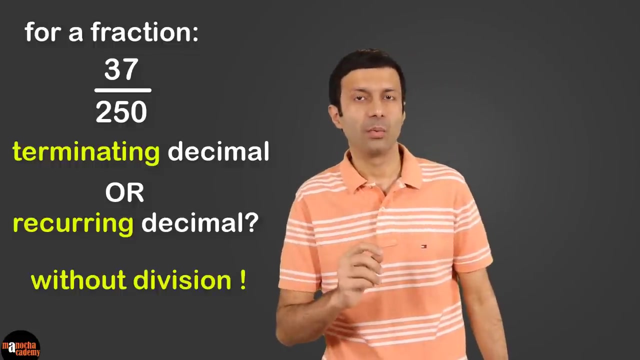 repeating. if you take any fraction, how do you determine that on division, you're going to get a terminating decimal number or a recurring decimal number? of course, one simple way is to actually do the division, but there's another trick where you don't need to do it. if you don't need to do it, if you don't need to. 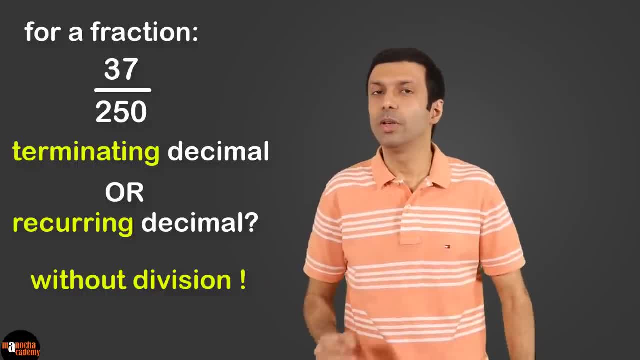 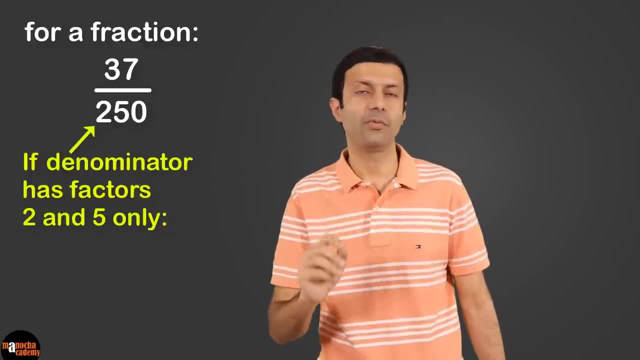 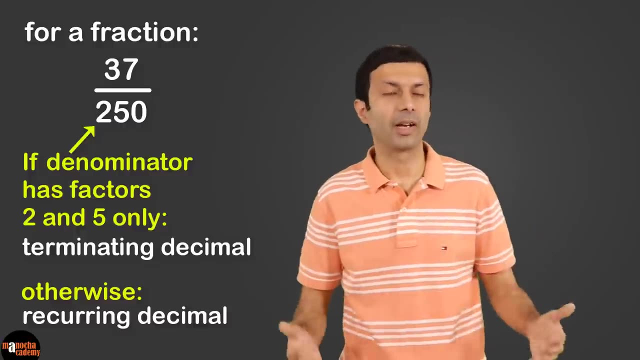 divide. now what's the trick? you need to take a look at the denominator, and if the denominator has factors of 2 and 5, only then you're going to get a terminating decimal number. otherwise it's going to be a recurring decimal number. let me pull up some examples to illustrate this. let's start with the. 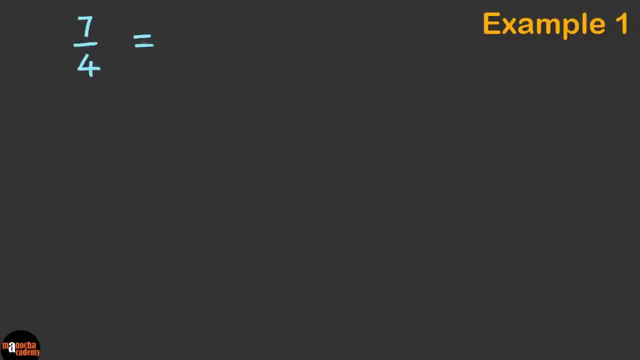 example of 7 by 4. now what are the factors of the denominator? for the denominator, it's 2 into 2. now our goal is to convert the denominator into multiples of tens, so I'm going to multiply 5 into 5 in the numerator and. 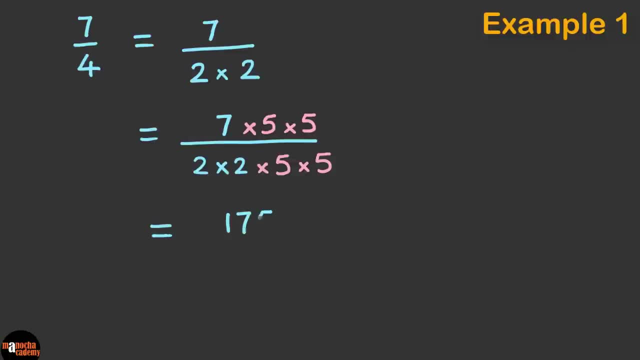 in the denominator. so I get 175 by 100, that's 1.75. so this is a terminating decimal number. but if we take 37 by 150, so what are the factors of the denominator? they are 2 into 3 into 5 into 5, and if you divide we get 0.24666 and so on. so 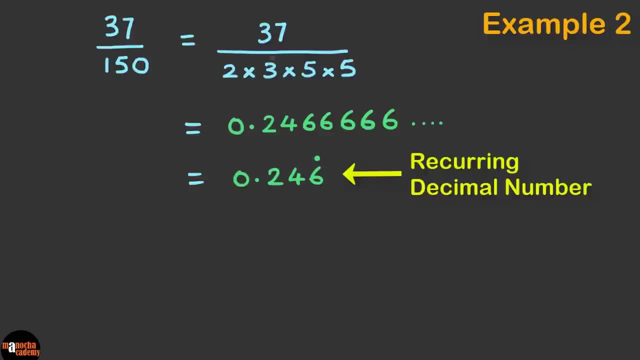 this is a recurring decimal number. and why is that? because if you carefully look at the factors in the denominator, you can see that there's a 3 there. for it to be a terminating decimal number, you need factors of 2 and 5, only now a. 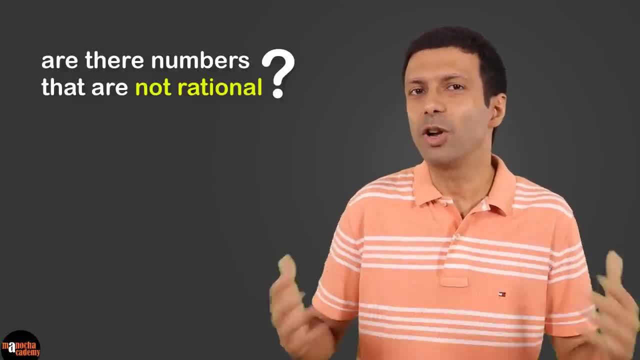 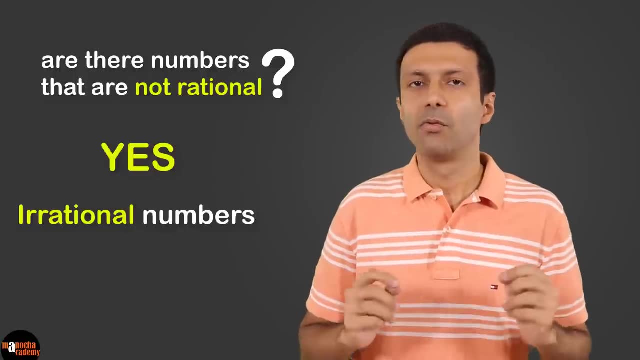 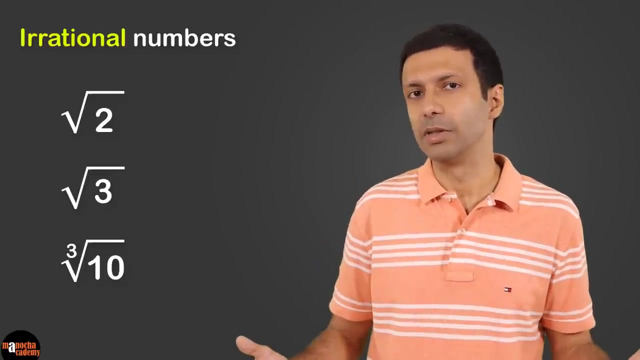 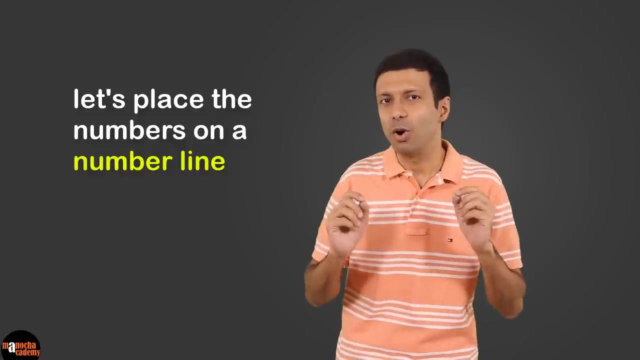 rational question is: are there numbers that are not rational? the answers yes. these are called irrational numbers. for example, root 2, root 3, cube, root of 10. these are all irrational numbers, but we look at these in a separate video. let's try to place the different numbers that we've learned on a number line are you familiar with. 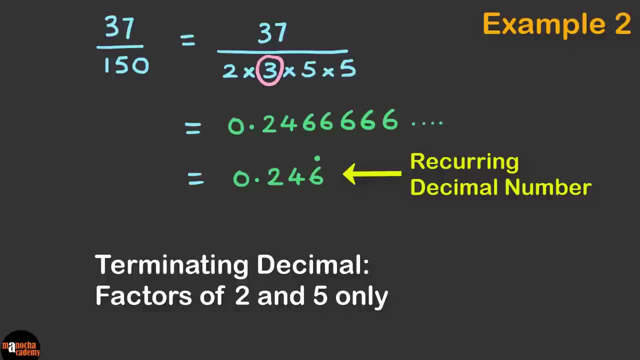 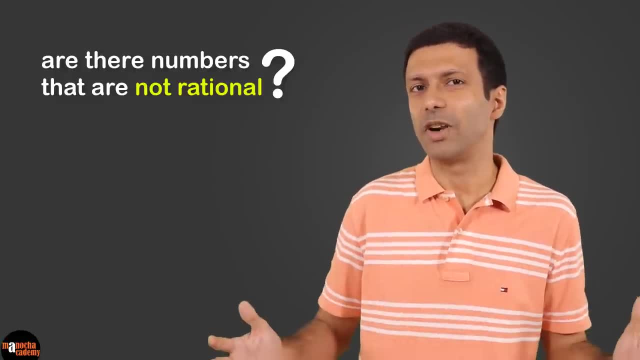 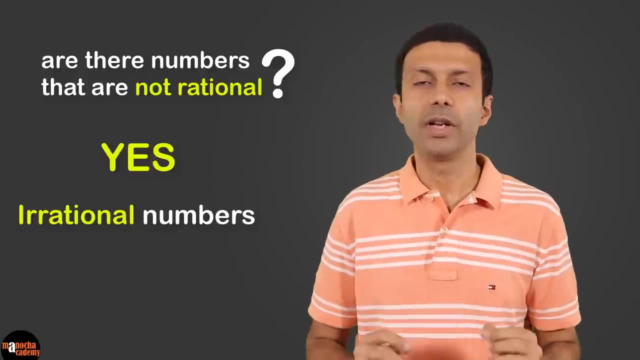 it to be a terminating decimal number, you need factors of 2 and 5 only now. a rational question is: are there numbers that are not rational? the answers yes. these are called irrational numbers. for example, root, 2, root, 3, cube, root of 10. these are all. 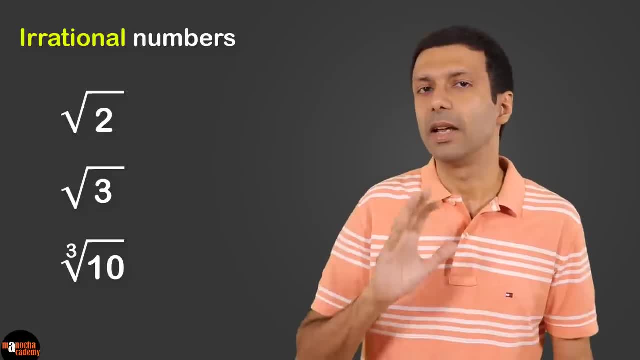 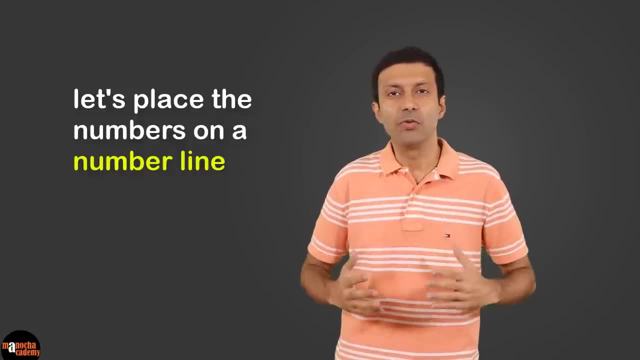 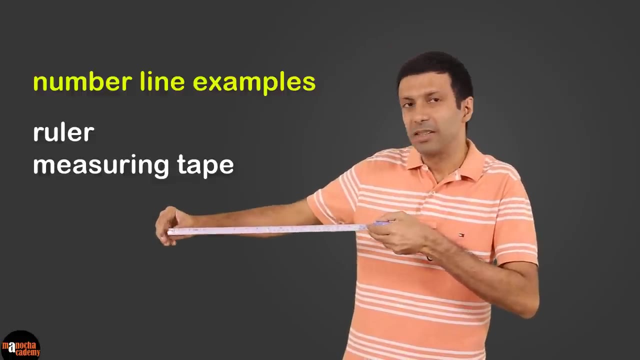 irrational numbers, but we look at these in a separate video. let's try to place the different numbers that we've learned on a number line. are you familiar with the number line? an everyday example is a ruler or a measuring tape like this with numbers marked on it. unlike the measuring, 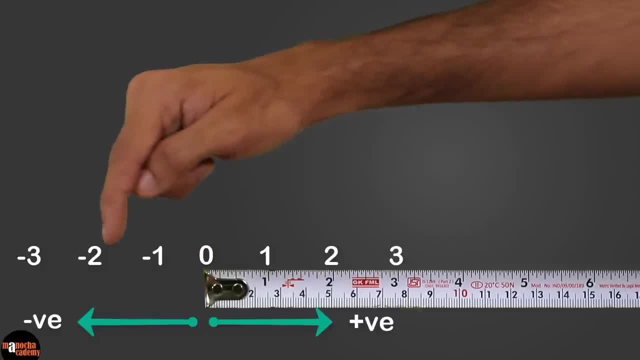 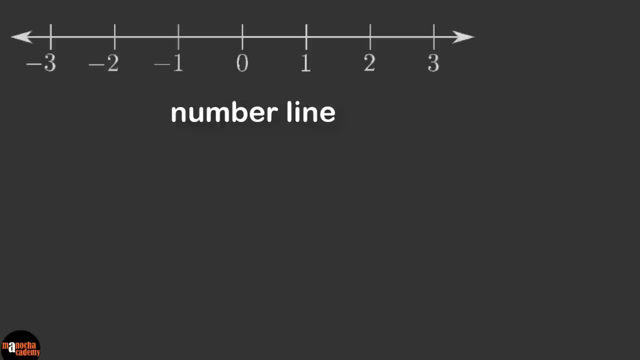 tape. the number line has both positive and negative numbers. so let's draw a number line and try to place the different numbers on it. so here's our number line. let's mark the natural numbers on it: 1, 2, 3 and so on. let's draw. 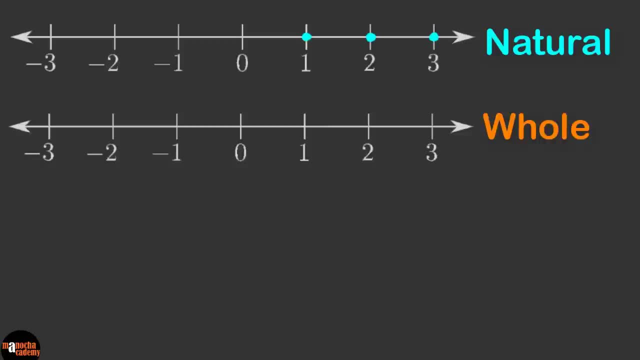 another number line and mark the whole numbers on it, so it's going to be the natural numbers and 0. in our third number line let's mark the integers, so it's going to be all the whole numbers and the negative numbers minus 1, minus 2, minus 3, and so on. in the next number line let's mark the rational. 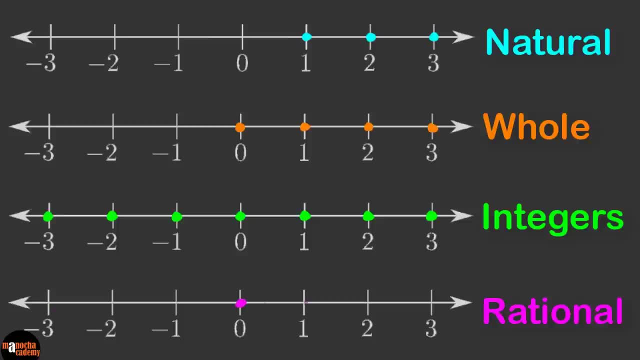 numbers, so it's going to be all the integers and decimals and fractions. for example, 1.5 is here, midway between 1 and 2, 2.8 is here and it's closer to 3, and minus half is midway between 0 and minus 1. we can also visualize the number. 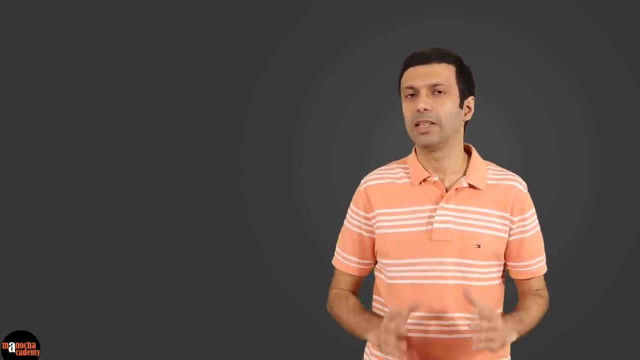 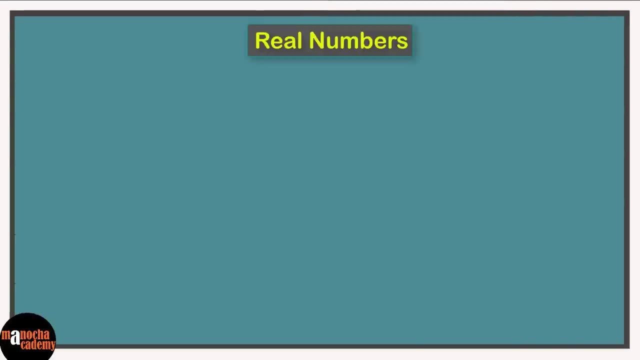 system by starting from the top, that is, from the real numbers. let me pull up the concept board for you. real numbers can be divided into rational and irrational numbers. rational numbers can be divided into integers and non integers. now, integers can be divided into negative integers and whole numbers. 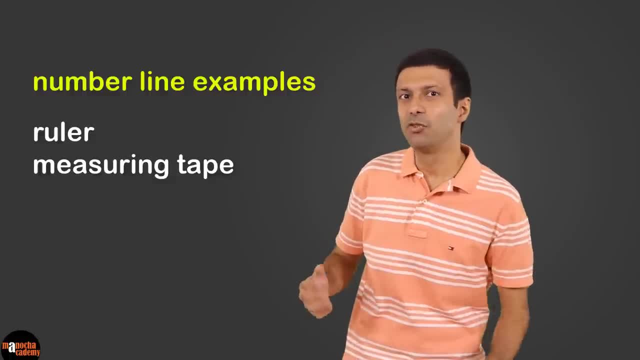 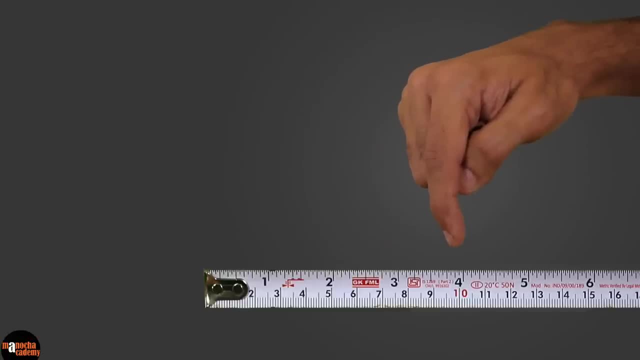 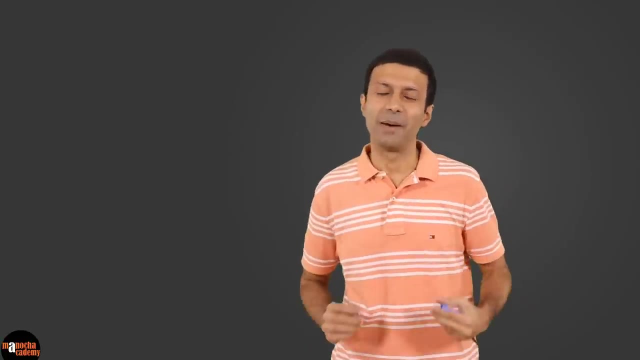 the number line. an everyday example is a ruler or a measuring tape like this with numbers marked on it. unlike the measuring tape, the number line has both positive and negative numbers. so let's draw a number line and try to place the different numbers on it. so here's our 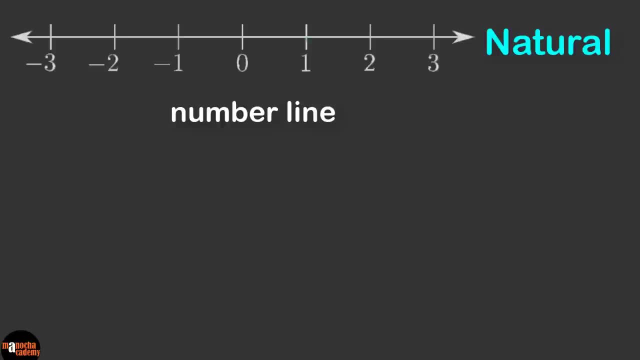 number line, let's mark the natural numbers on it: one, two, three and so on. let's draw another number line and mark the whole numbers on it. it, So it's going to be the natural numbers and 0.. In our third number line, let's mark: 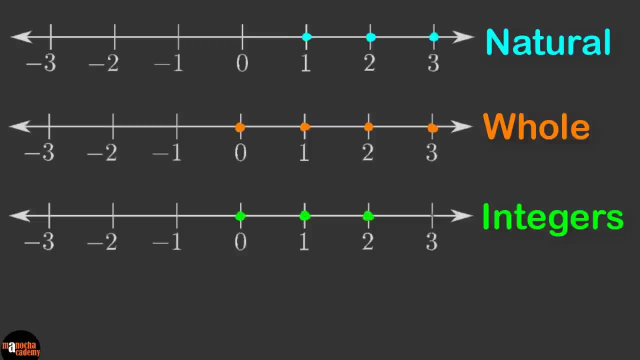 the integers, So it's going to be all the whole numbers and the negative numbers Minus 1,, minus 2, minus 3 and so on. In the next number line let's mark the rational numbers, So it's going to be all the integers and decimals and fractions. For example, 1.5 is 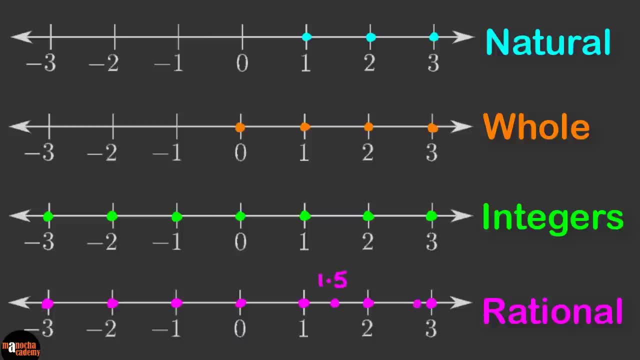 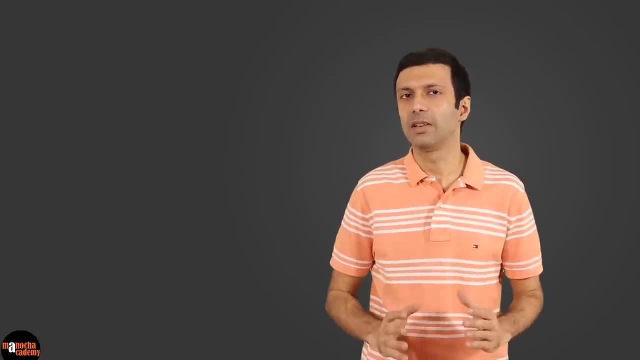 here midway between 1 and 2.. 2.8 is here and it's closer to 3. And minus half is midway between 0 and minus 1.. We can also visualize the number system by starting from the top, that is, from the real numbers. 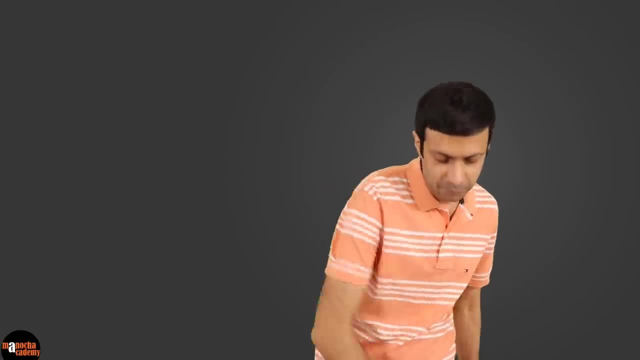 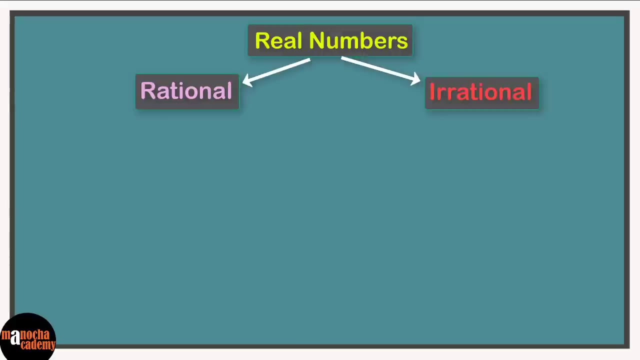 Let me pull up the concept board for you. Real numbers can be divided into rational and irrational numbers. Rational numbers can be divided into integers and non-integers. Now integers can be divided into negative integers and whole numbers. Whole numbers can be split into 0 and positive. 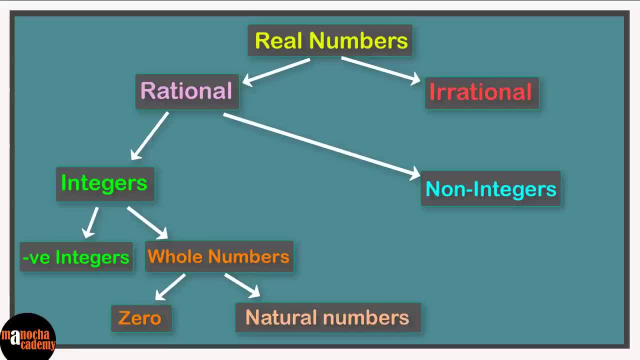 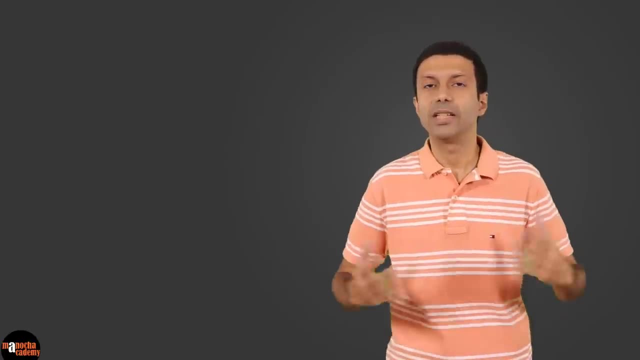 integers, which are natural numbers. Coming back to the non-integers, fractions and decimals. These can be divided into terminating decimals and non-terminating or recurring decimals. Now let's say you want to find rational numbers between any two given rational numbers For 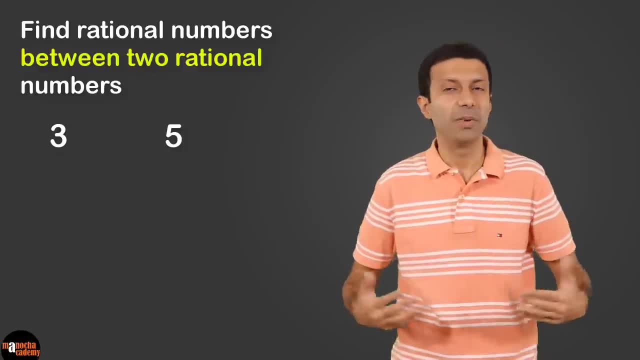 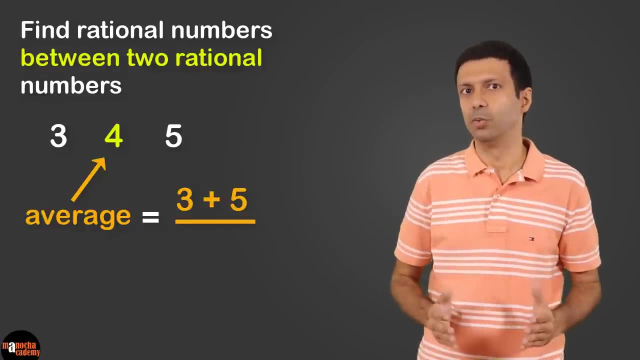 example, between 3 and 5.. One simple answer is 4.. We can get it by finding the average 3 plus 5. By 2. Which is equal to 4.. If you want to find more rational numbers, then you can do 3 plus 4. 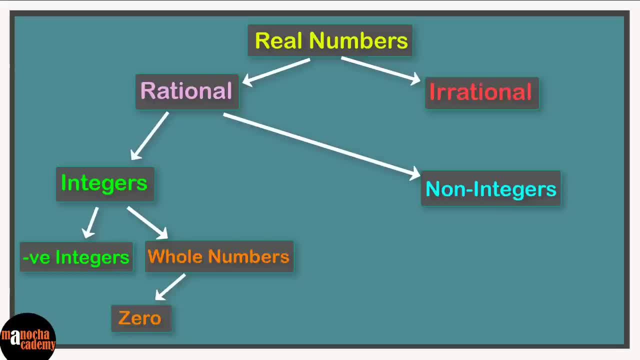 whole numbers can be split into 0 and positive integers, which are natural numbers. coming back to the non integers, fractions and decimals, these can be divided into terminating numbers and non-integers. these can be divided into decimals and non-terminating or recurring decimals. now let's say you want to find 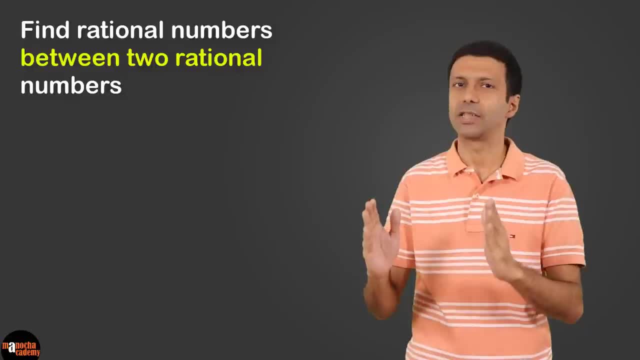 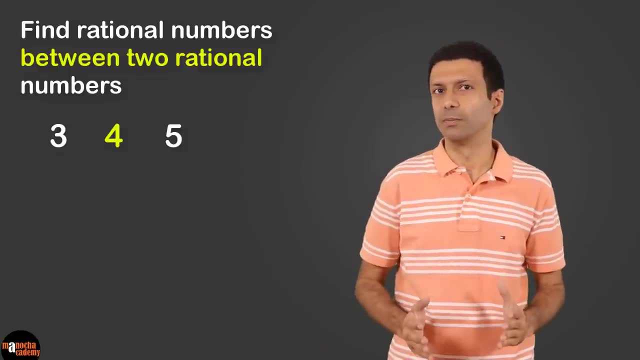 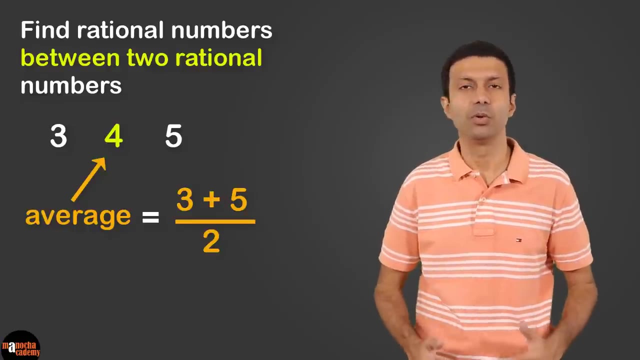 rational numbers. between any two given rational numbers, for example between 3 and 5, one simple answer is 4. we can get it by finding the average 3 plus 5 by 2, which is equal to 4. if you want to find more rational numbers, then you can do 3. 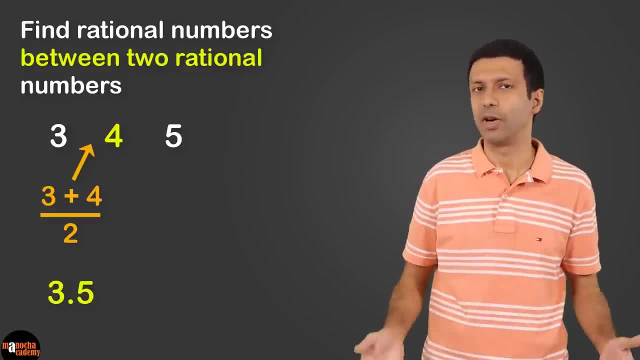 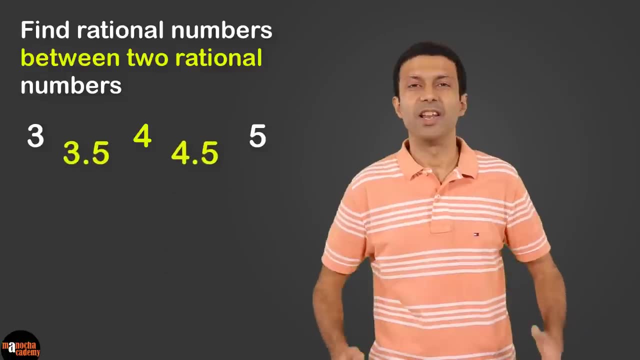 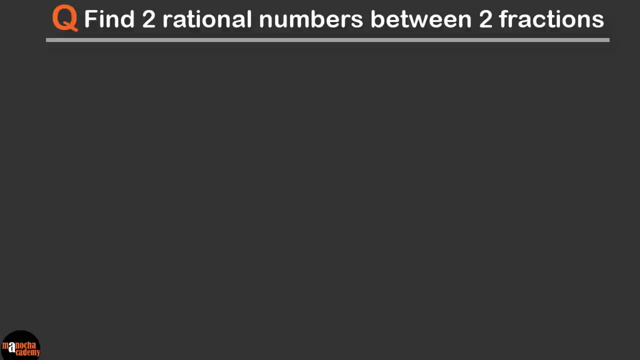 plus 4 by 2, that's 3.5, and 4 plus 5 by 2, which is 4.5. now let me pull up some more interesting examples for you. if you want to find two rational numbers between two fractions, for example 1 by 7 and 4 by 7, since the denominators here are equal and the numerators 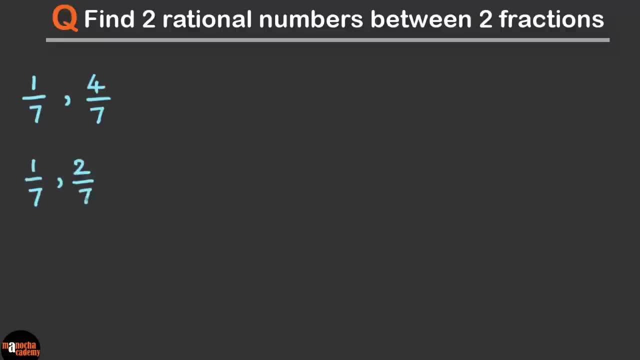 have a gap, we can fill in the fractions in the gap. so our answer is going to be 2 by 7 and 3 by 7. but what if there's no gap? for example, if we have to find two rational numbers between 1 by 7 and 2 by 7, then what do you do? we can create a gap by 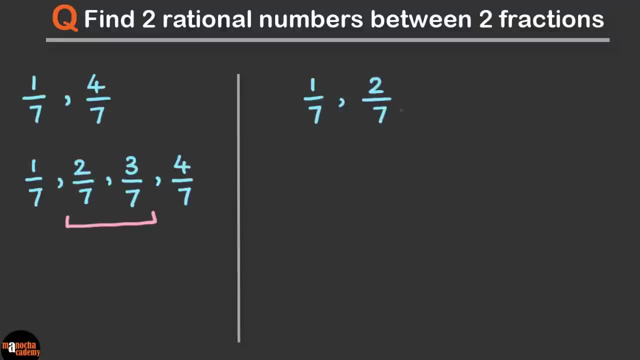 multiplying the numerator and denominator with a number. since we need two rational numbers, we will multiply by 2 plus 1, which is 3. multiplying the numerator and denominator of the two fractions by 3, we get 3 by 21 and 6 by 21. again, the denominators are the same. 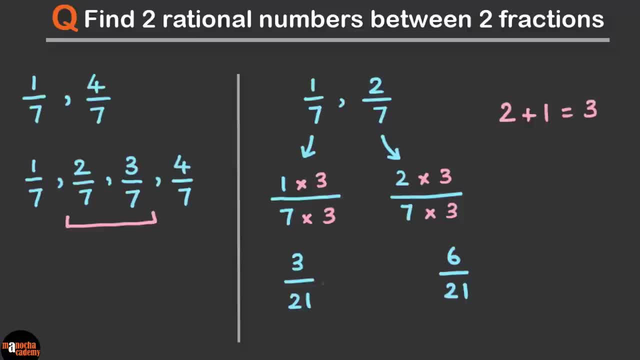 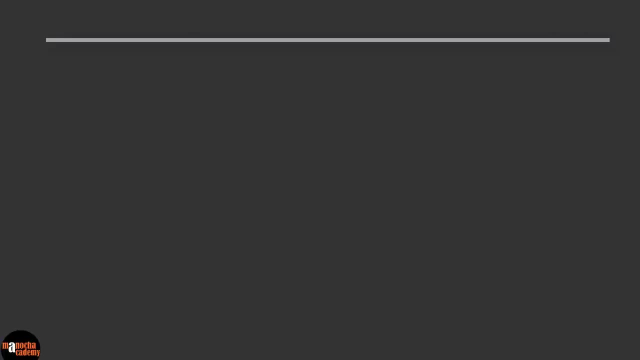 but can you see that we've got a gap in the numerator. so the two fractions we can insert are 4 by 21 and 5 by 21. now let's look at the case with the denominators of the two fractions are not the same. for example, if we want to insert six rational numbers between: 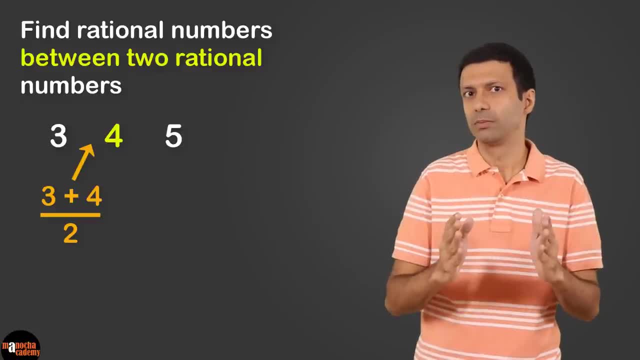 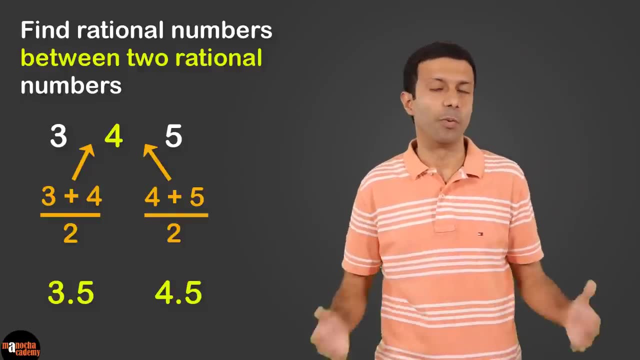 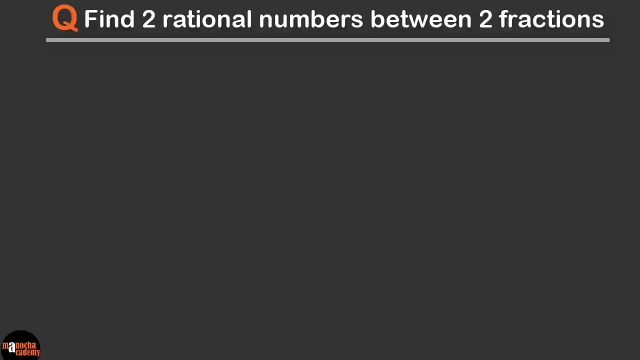 by 2,, that's 3.5.. And 4 plus 5 by 2, which is 4.5.. Now let me pull up some more interesting examples for you, If you want to find two backwards rational numbers between two fractions. 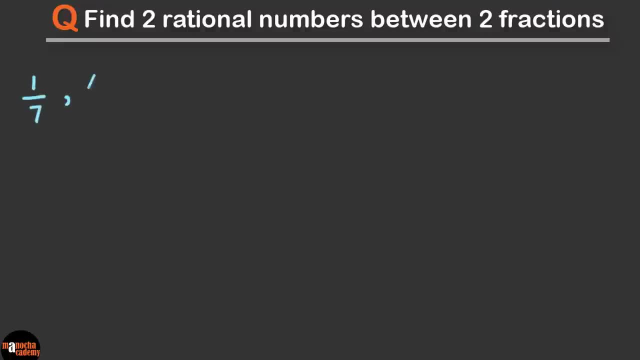 For example, hurt matters. Listen carefully: 1 and 5.. 1 by 7 and 4 by 7.. Since the denominators here are equal and the numerators have a gap, we can fill in the fractions in the gap. 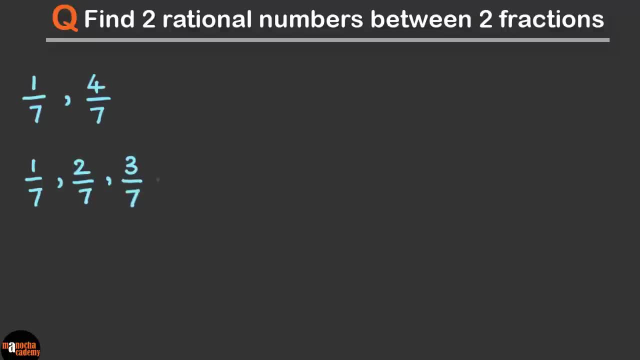 So our answer is going to be 2 by 7 and 3 by 7.. But what if there is no gap, For example, if we have to find two rational numbers between 1 by 7 and 2 by 7,? 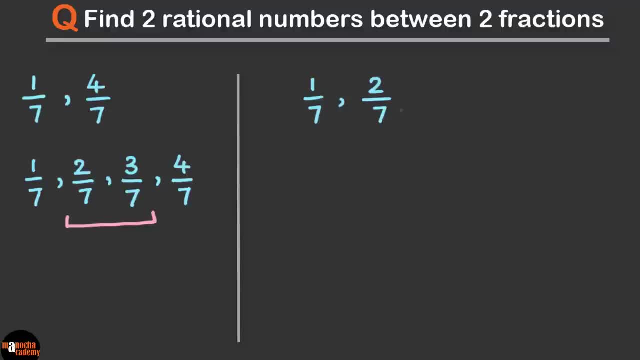 then what do you do? We can create a gap by multiplying the numerator and denominator with a number. Since we need two rational numbers, we will multiply by 2 plus 1, which is 3.. Multiplying the numerator and denominator of the two fractions by 3,. 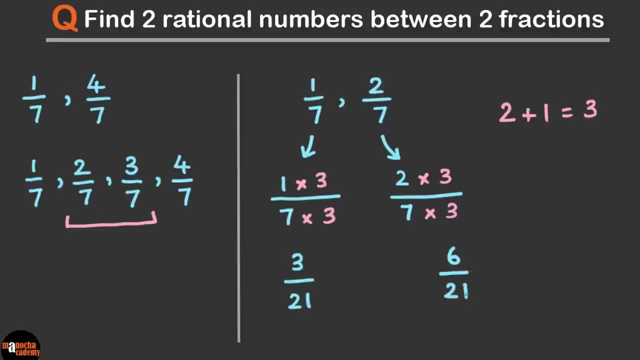 we get 3 by 21 and 6 by 21.. Again, the denominators are the same, But can you see that we've got a gap In the numerator? so the two fractions we can insert are 4 by 21 and 5 by 21.. 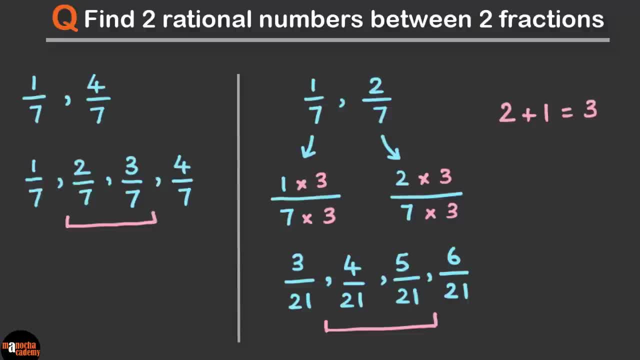 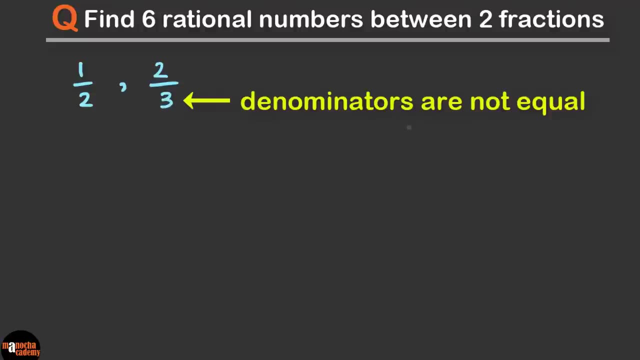 Now let's look at the case where the denominators of the two fractions are not the same. For example, if we want to insert six rational numbers between half and two-third, As you can see, the denominators are not equal. So the first step is to make the denominators equal. 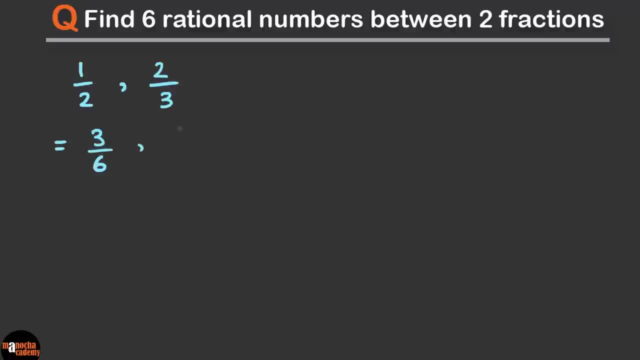 So our two fractions become 3 by 6 and 4 by 6.. Similar to our previous case. now the two denominators are equal, but there is no gap in the numerators. So what should we do? That's right, we need to multiply by a number. 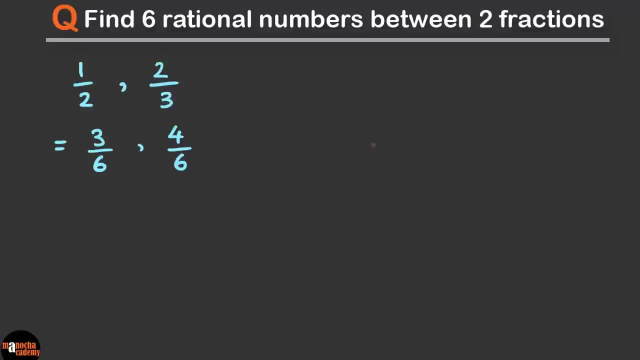 And since we need to insert six rational numbers, our number is going to be 6 plus 1, which is 7.. So let's multiply the numerator and denominator. So here we have 21 by 42 and 28 by 42.. 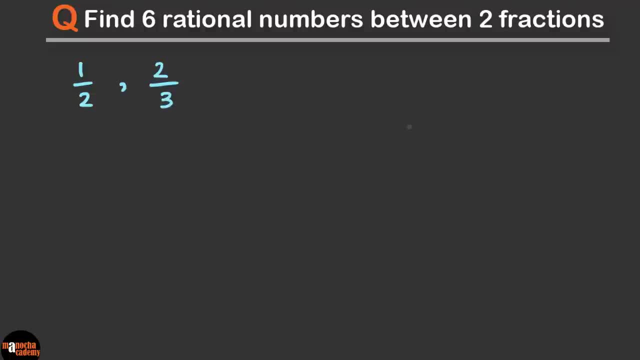 half and two-thirds. as you can see, the denominators are not equal. so the first step is to make the denominators equal. so our two fractions become 3 by 6 and 4 by 6, similar to a previous case. now the two denominators are equal, but there's no. 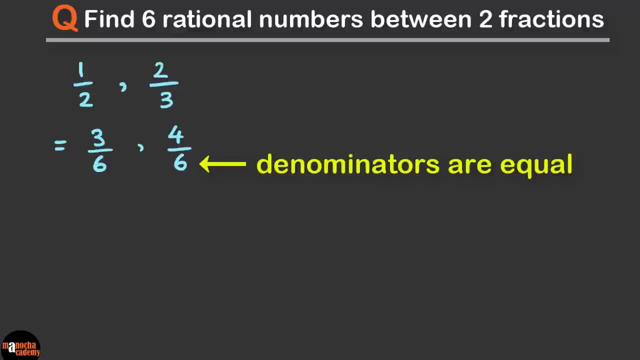 gap in the numerators. so what should we do? that's right, we need to multiply by a number and since we need to insert six rational numbers, our number is going to be 6 plus 1, which is 7. so let's multiply the numerator and denominator of the two. 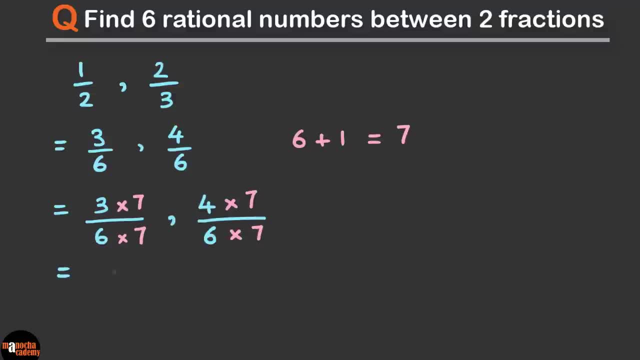 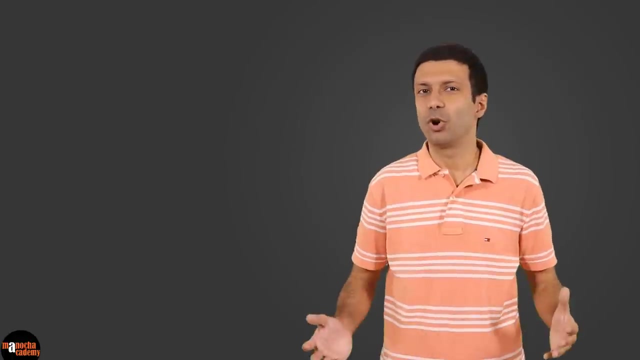 fractions by 7. so here we have 21 by 42 and 28 by 42. so here are the six rational numbers that we can insert between these two fractions and on simplifying the six rational numbers, and that's our answer. let's talk about fractions and decimals, how to convert fractions to decimals and 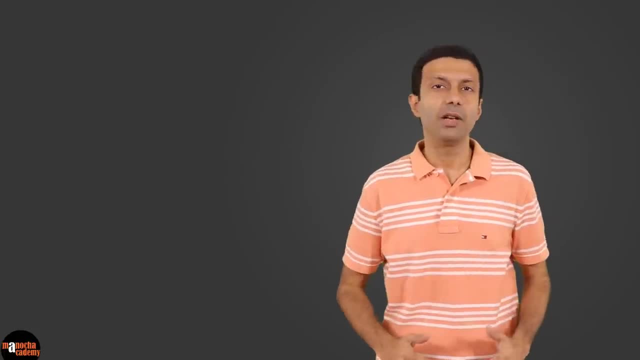 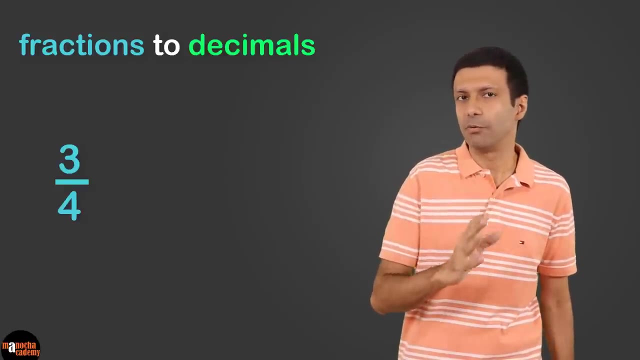 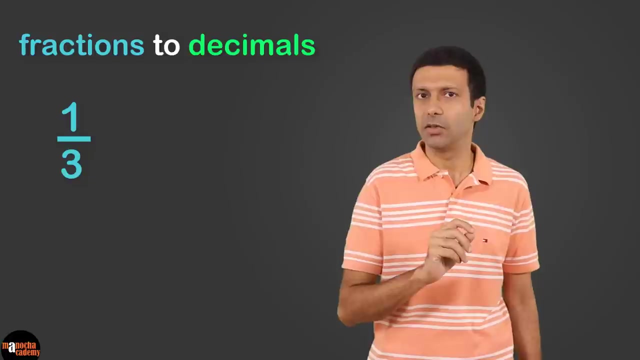 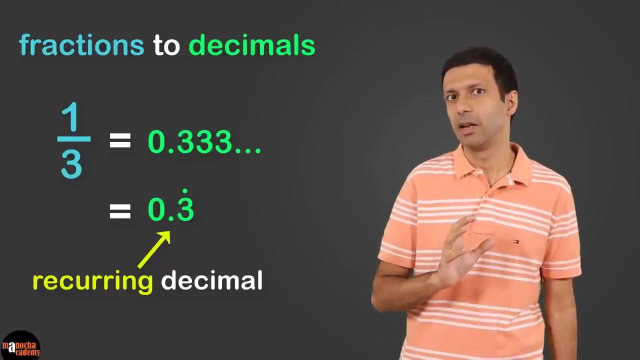 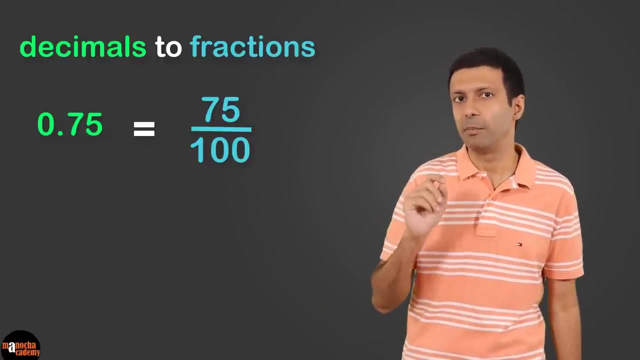 decimals to fractions. converting fractions to decimals is easy. you just need to divide. For example, 3 by 4 is 0.75, a terminating decimal number. 1 by 3 is 0.333, recurring a recurring decimal number. Now, if you want to convert 0.75 to a fraction, then we can write it as 75 by 100.. 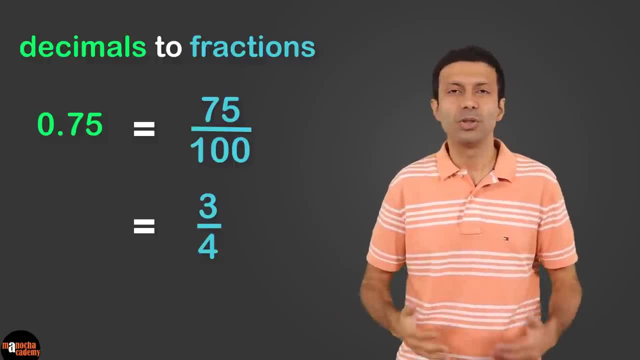 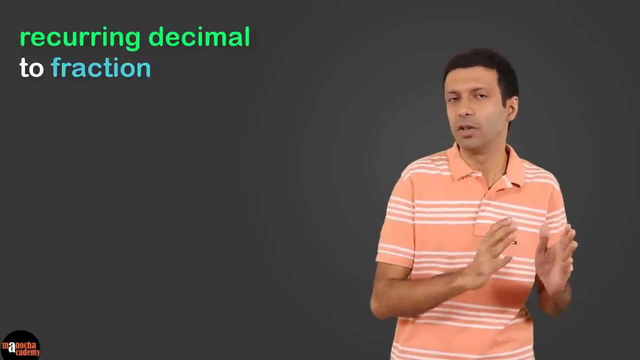 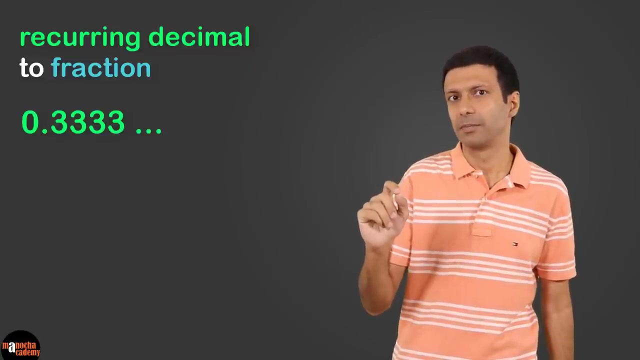 Simplifying, we get 3 by 4.. So these are simple. But a more interesting question is: how do you convert a recurring decimal number to a fraction, For example, 0.333 recurring. Now we know that 0.3 is 3 by 10.. 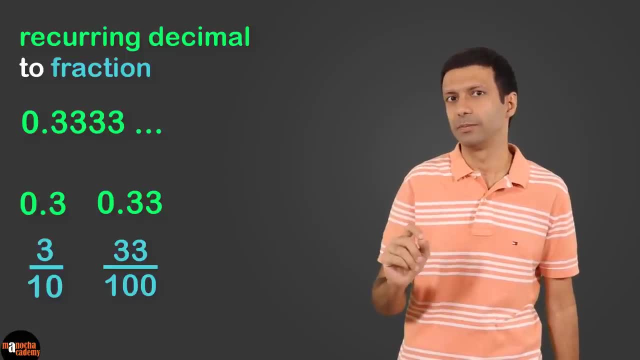 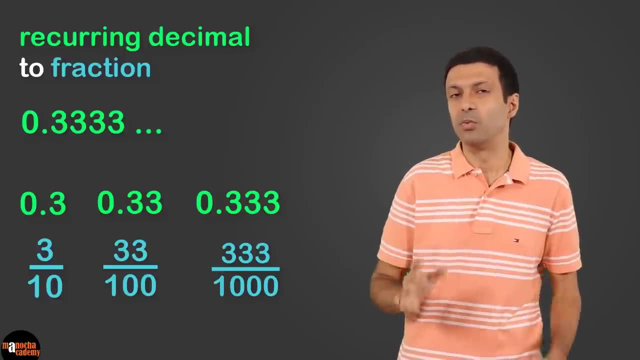 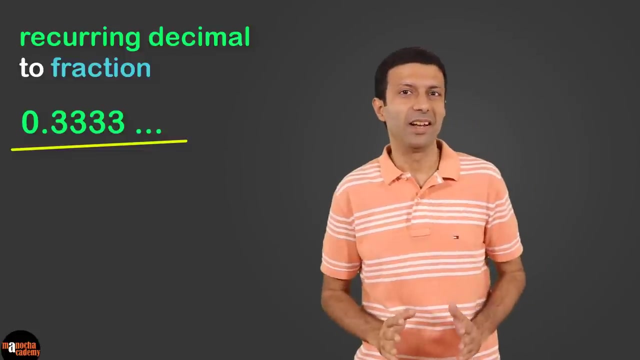 0.33 is 33 by 100.. 0.333 is 333 by 1000.. But we are looking for 0.333.. So let me show you the technique: how to convert a recurring decimal number to a fraction. 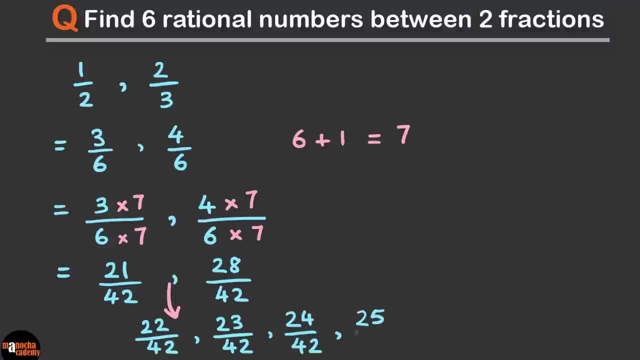 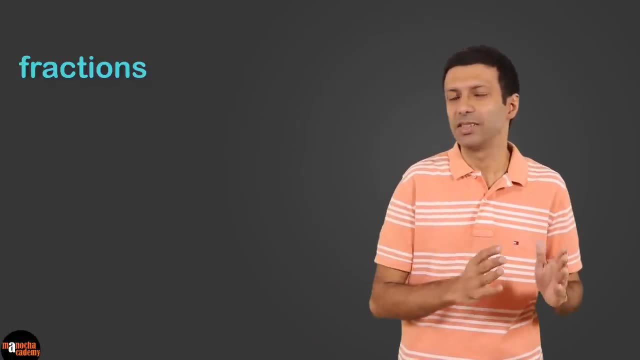 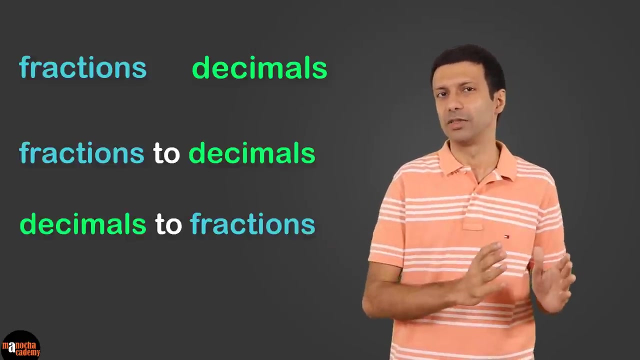 So here are the six rational numbers that we can insert between these two fractions. And on simplifying the six rational numbers- and that's our answer- Let's talk about fractions and decimals, How to convert fractions, So you can convert fractions to decimals and decimals to fractions. 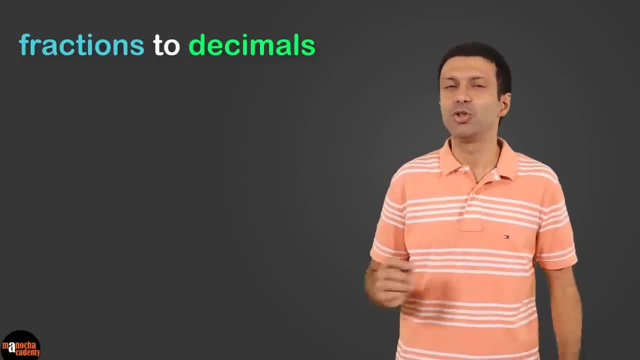 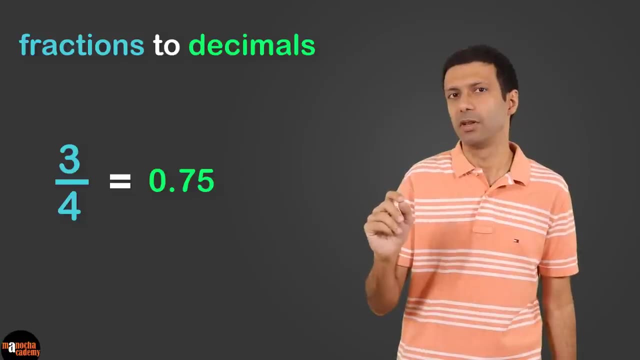 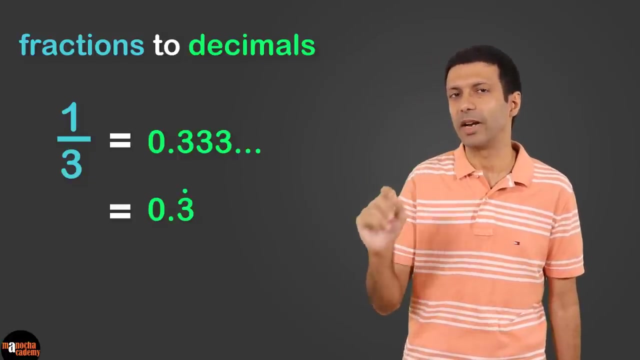 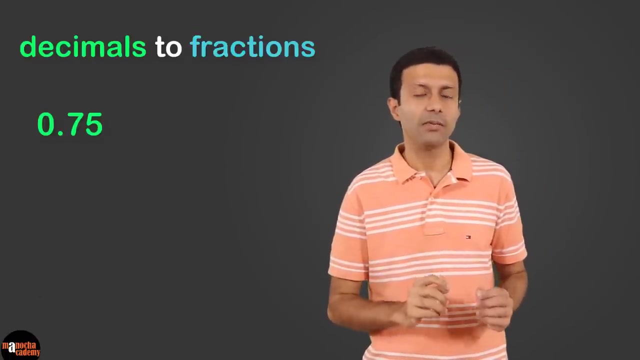 Converting fractions to decimals is easy. You just need to divide. For example, 3 by 4 is 0.75, a terminating decimal number. 1 by 3 is 0.333- recurring a recurring decimal number. Now, if you want to convert 0.75 to a fraction, 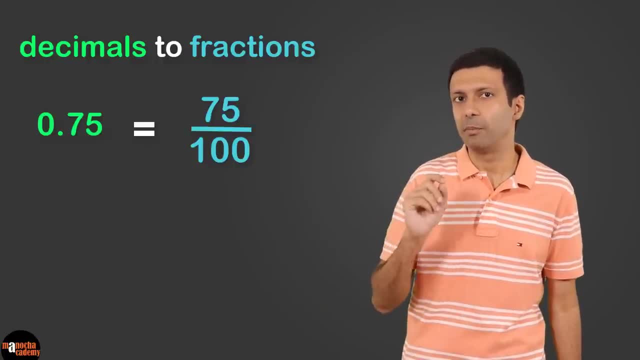 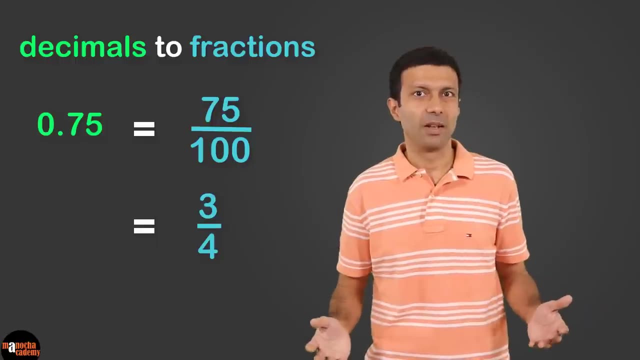 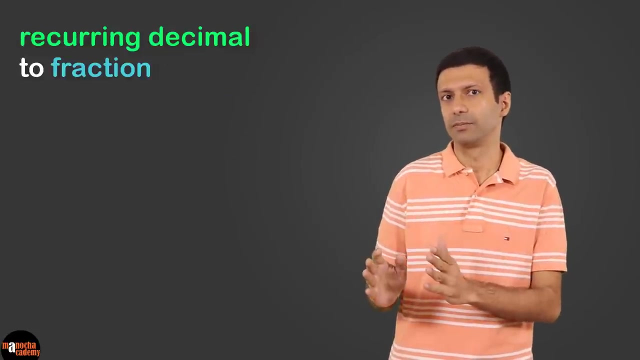 then we can write it as 75 by 100.. Simplifying, we get 3 by 4.. So these are simple. But a more interesting question is how do you convert a recurring decimal number to a fraction, For example, 0.333 recurring. 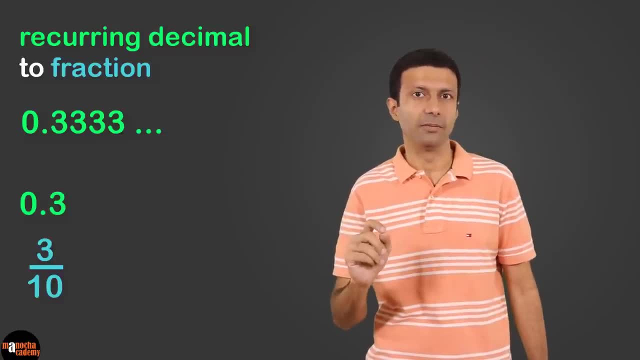 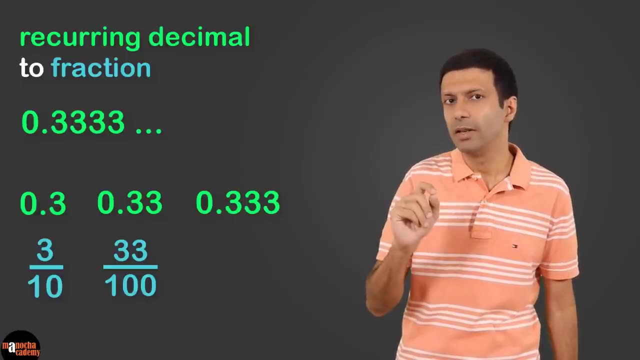 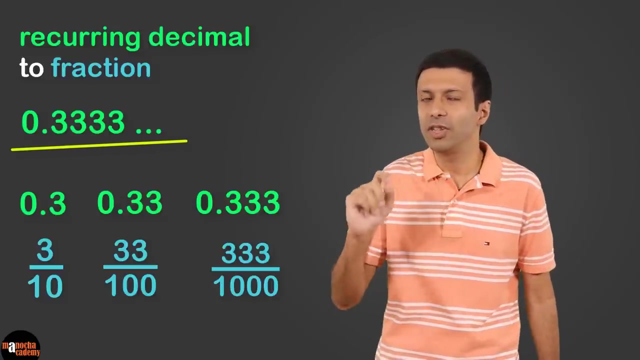 Now we know that 0.3 is 3 by 10.. 0.33 is 30.. 0.333 is 33 by 100.. 0.333 is 333 by 1000.. But we are looking for 0.3333 recurring. 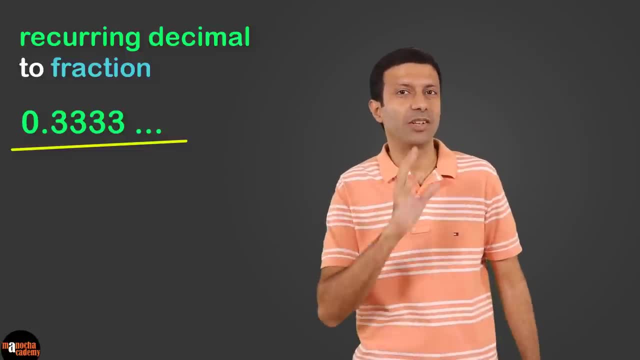 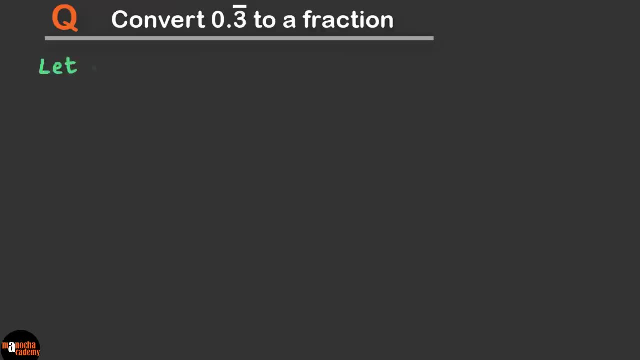 So let me show you the technique: how to convert a recurring decimal number to a fraction Coming up for you right now. Let x be the recurring decimal number, which is 0.3 recurring in this case. So let's write it as x. 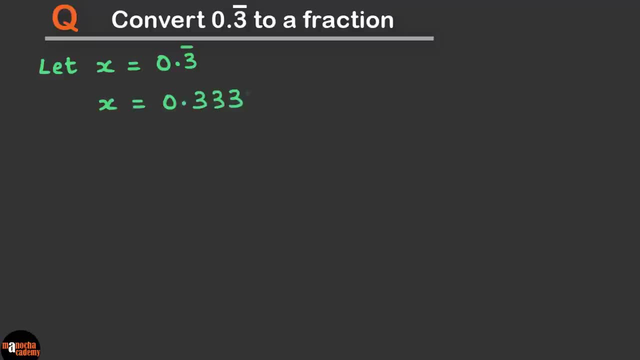 Let x, equal to 0.3333, and so on. Now we need another number where the part after the decimal is the same. So let's multiply x by 10. And we have 10x equal to 3.333, and so on. 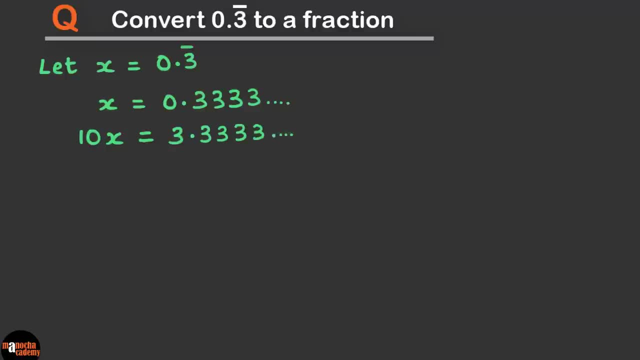 So, as you can see here, x and 10x have the same part after the decimal. Now let's subtract x from 10x. So I'm going to copy the first line here: On subtracting, we get 9x equal to 3.. 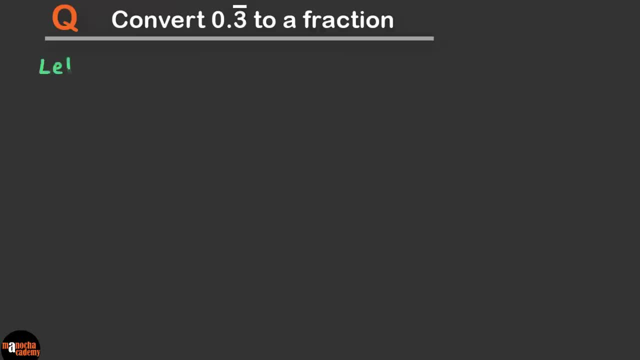 Coming up for you right now. Let x be the recurring decimal number, which is 0.3- recurring in this case. So let's write it as x equal to 0.3333, and so on. Now we need another number where the part after the decimal is the same. 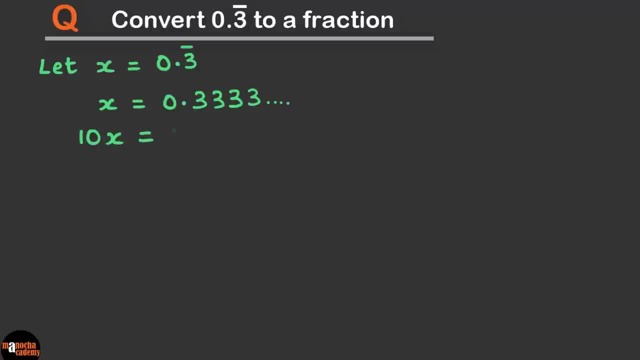 So let's multiply x by 10 and we have 10x equal to 3.333, and so on. So as you can see here, x and 10x have the same part after the decimal. Now let's subtract x from 10x. 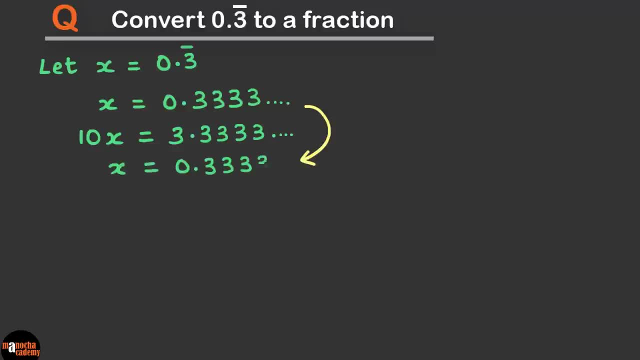 So I'm going to copy the first line here. On subtracting, we get 9x equal to 3.. So x is 3 by 9.. And if we simplify we get 1 by 3.. So we have converted our recurring decimal number, 0.3 recurring, to a fraction 1 by 3.. 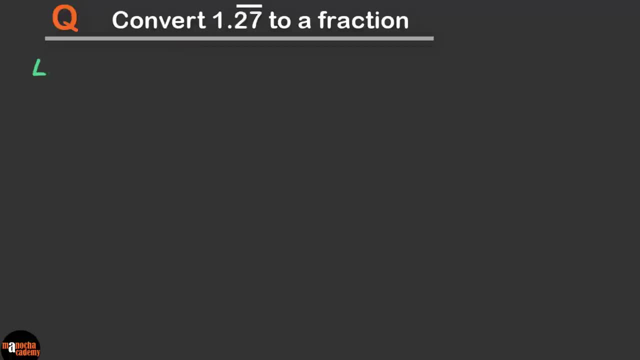 Let's look at another example Again. let x be the recurring decimal number, which is 1.27, recurring To find another number with the decimal part matching. this time we can't multiply by 10. We need to multiply by 100. 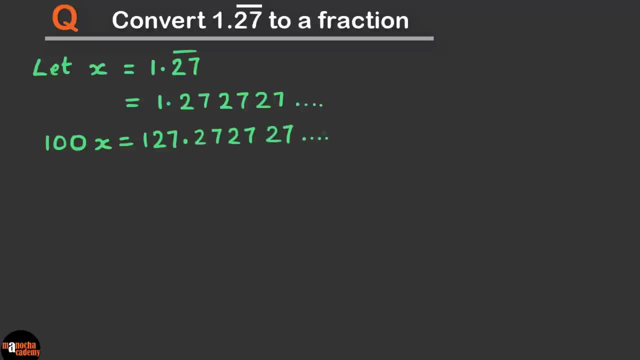 And, as you can see, in 100x the decimal part matches. So once again, subtracting x from 100x, we get 99x equal to 126. And on simplifying, we get 14 by 11.. 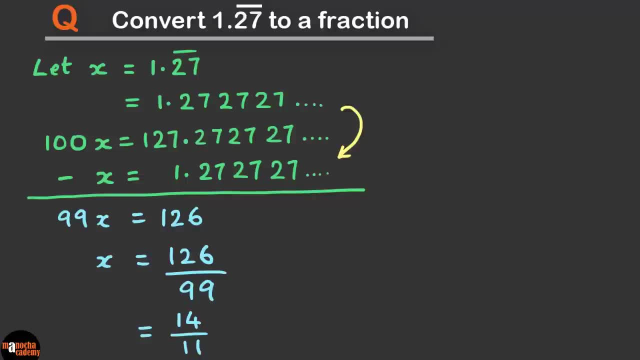 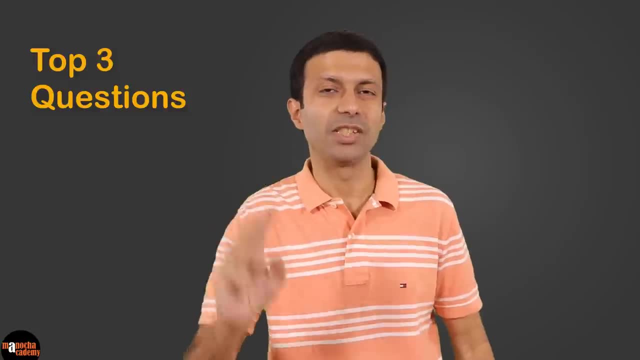 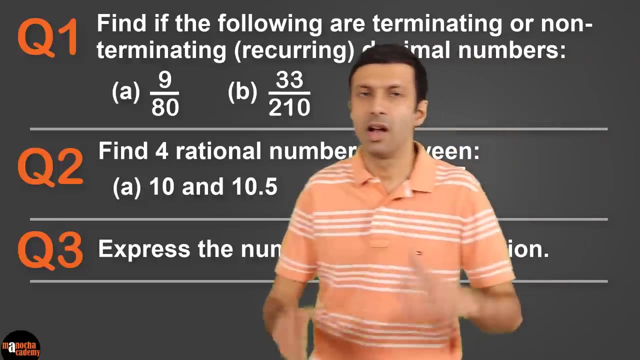 So we've converted our recurring decimal number to a fraction. Now that we are done with the topic of rational numbers, let's take a look at the top three questions. Let's take a look at the top three questions, three questions on this topic coming up for you right now. I would like you to 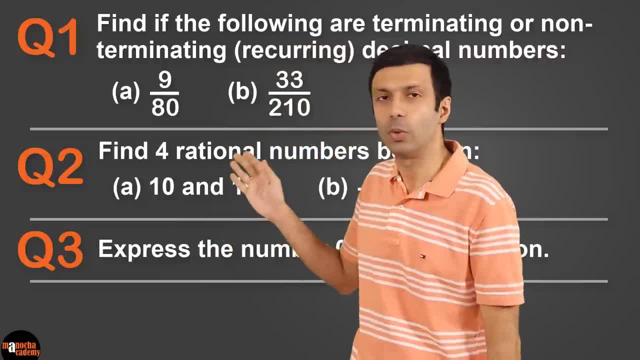 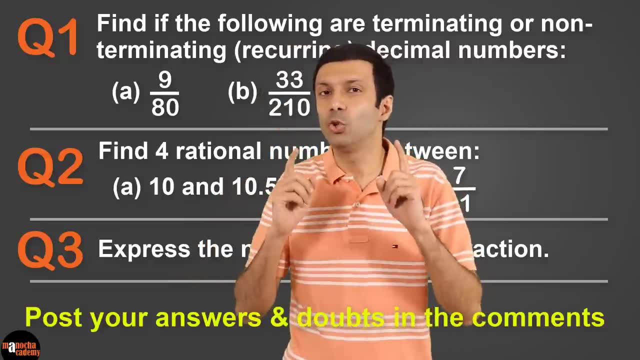 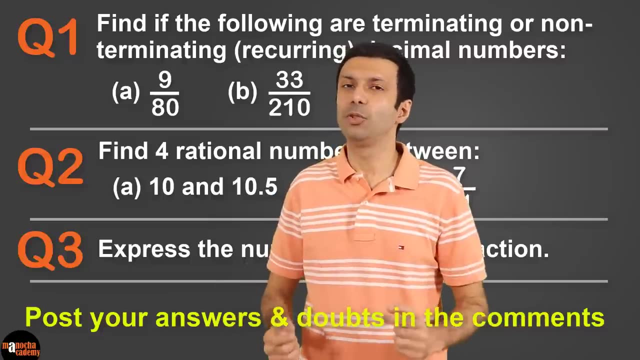 pause the video right here and try solving these questions. let's make this more interactive than just watching the video. so do post your answers in the comments below or, if you have any doubts, questions, feel free to write it in the comments below and I'm going to make a commitment to answer all of them. 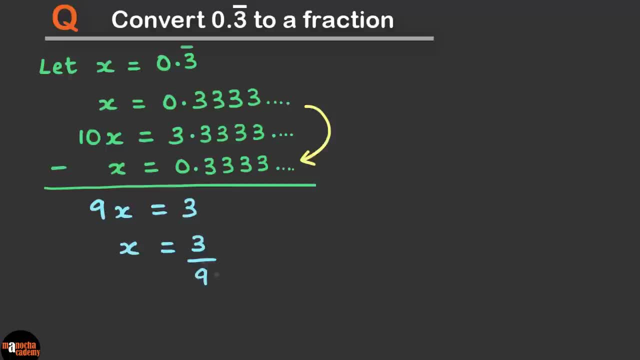 So x is 3 by 9.. And if we simplify we get 1 by 3.. So we have converted our recurring decimal number, 0.3 recurring, to a fraction 1 by 3.. Let's look at another example. 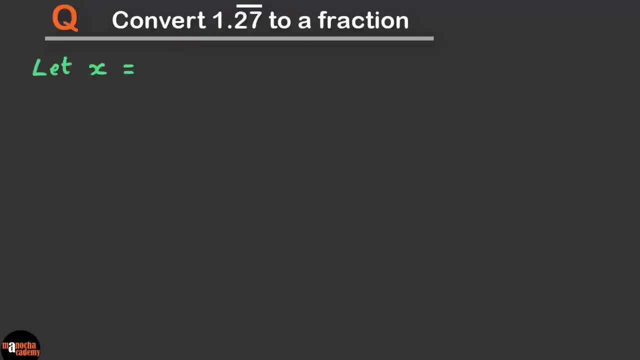 Again, let x be the recurring decimal number. Let x be the recurring decimal number which is 1.27, recurring To find another number with the decimal part matching. this time we can't multiply by 10. We need to multiply by 100. 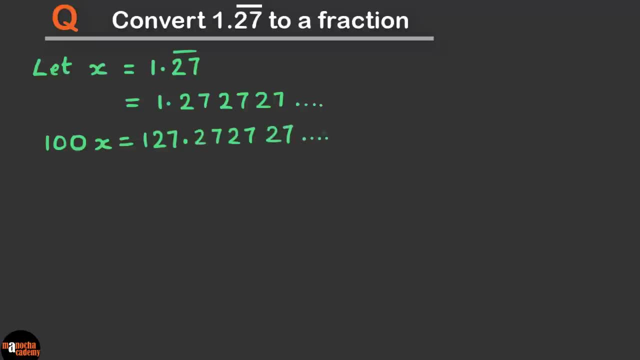 And, as you can see, in 100x the decimal part matches. So once again, subtracting x from 100x, we get 99x equal to 126. And on simplifying, we get 14 by 11.. 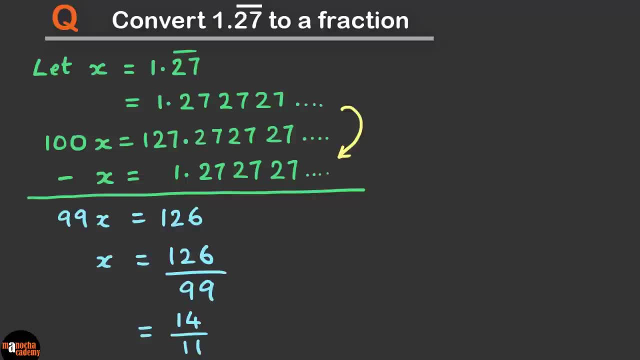 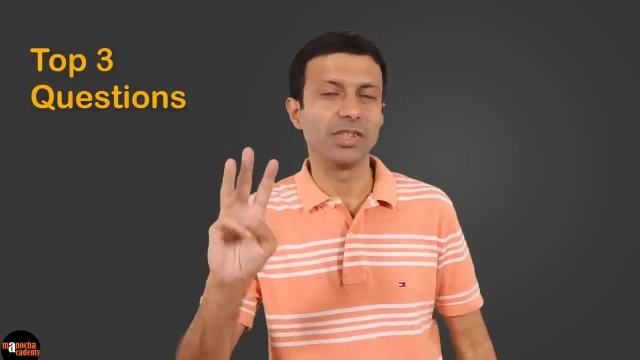 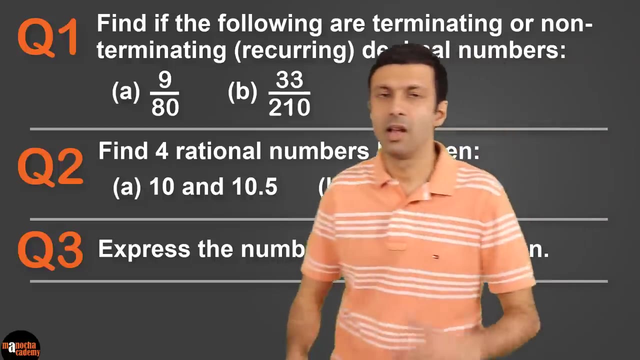 So we've converted our recurring decimal number to a fraction. Now that we are done with the topic of rational numbers, let's take a look at the top three questions on this topic Coming up for you right now. I would like you to pause the video right here and try solving these questions. 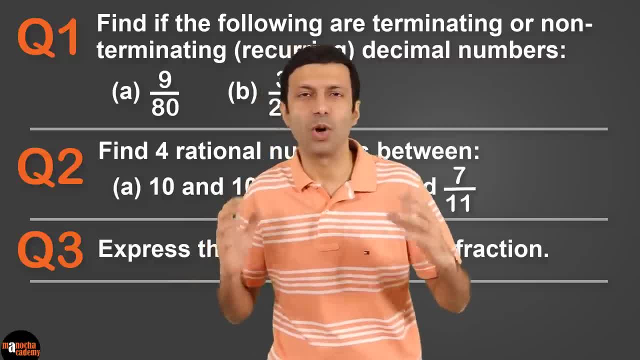 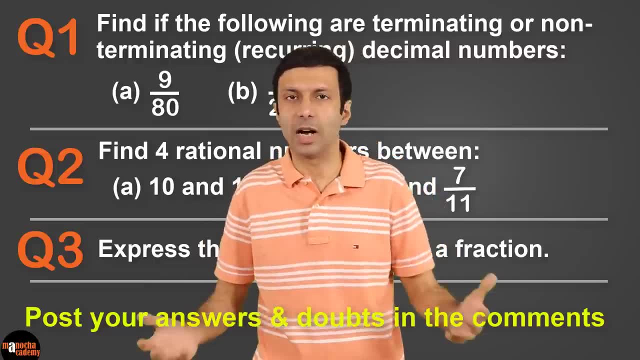 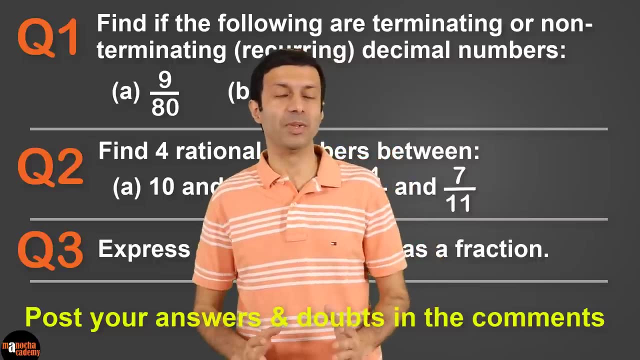 Let's make this more interactive, So do post your answers in the comments below, Or, if you have any doubts, questions, feel free to write it in the comments below, And I'm going to make a commitment to answer all of them promptly. 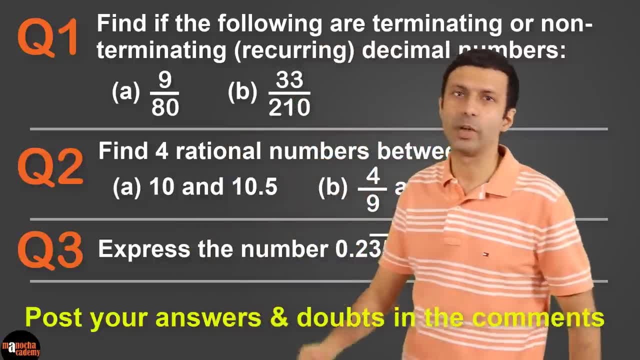 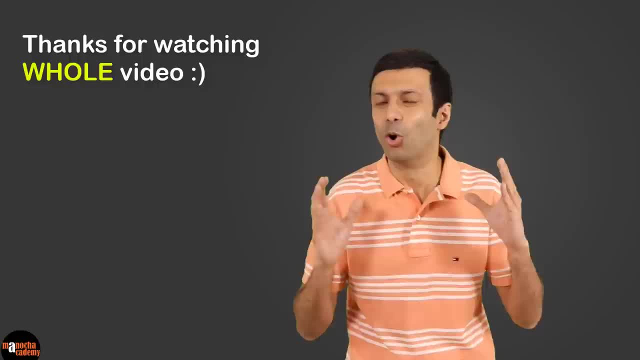 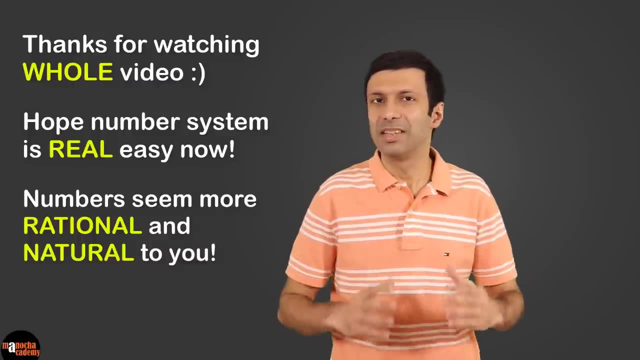 So I'm going to move off and let you solve these questions. Thanks for watching the whole video. I hope the number system is real easy for you now And the numbers seem more rational and natural to you. All puns intended in that sentence. 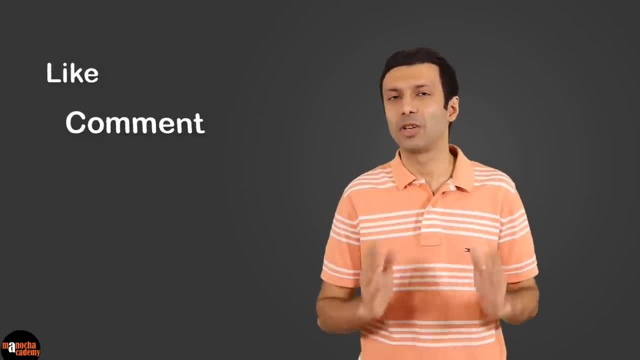 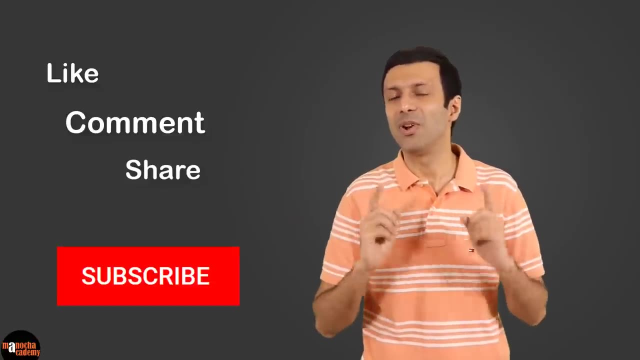 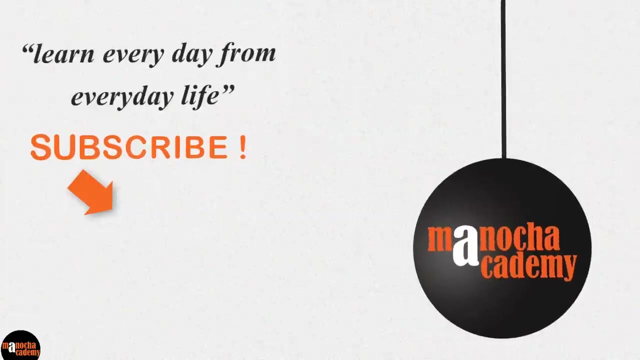 And do remember to like, comment and share out this video And go and hit the subscribe button for my channel right now. See you next time, Bye, bye.